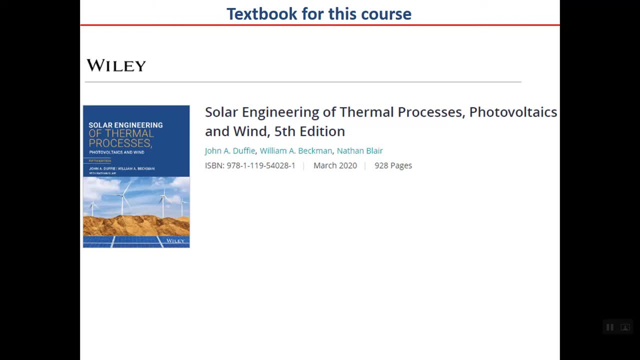 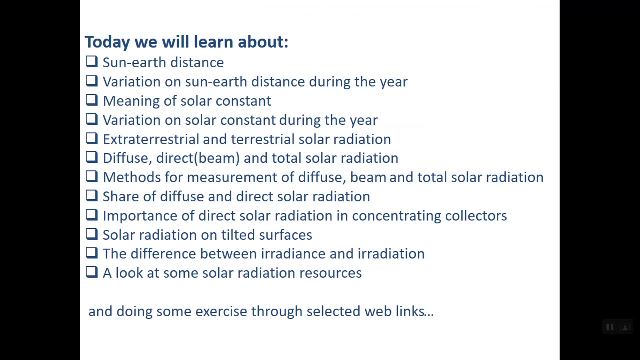 The textbook for our course is a very well known textbook: solar engineering of thermal processes. This is the fifth edition, actually in the new edition which has been published on 2020.. Some chapters are added regarding photovoltaics and wind also, So you can prepare the book. There are other references which I introduced you during the study. 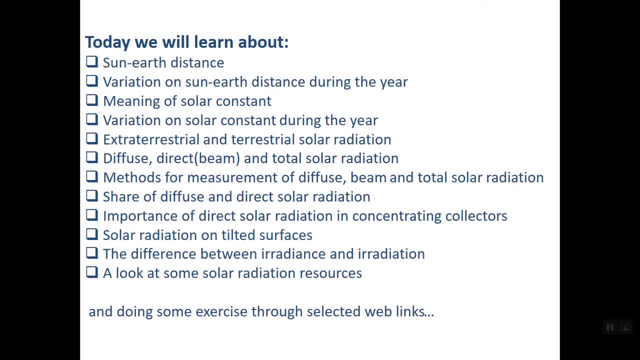 Today we will learn about the sun-earth distance, variation of solar energy, What is solar constant and its variation, The meaning of extraterrestrial and terrestrial solar radiation, Component of radiation- I mean diffuse and direct- And how to measure them. How to measure diffuse beam, direct and total solar radiation. 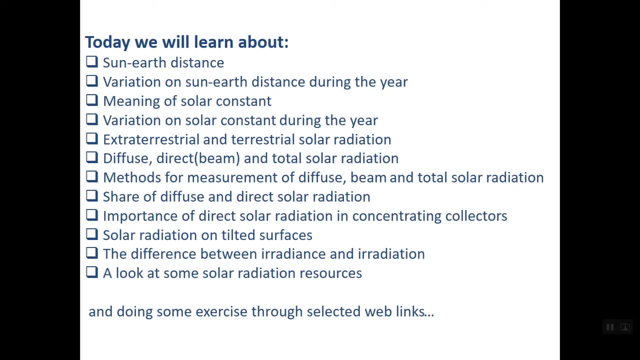 What are the share of diffuse and direct solar radiation And the importance of beam or direct radiation in concentrating collectors And an introduction to solar radiation on tilted surfaces, A very important definition about the difference between irradiance and irradiation or insulation, And we will look together at some solar radiation resources. 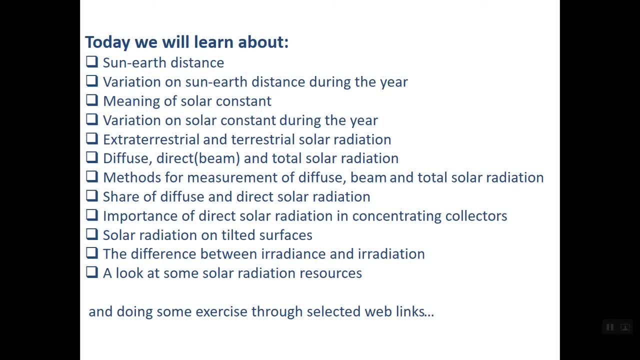 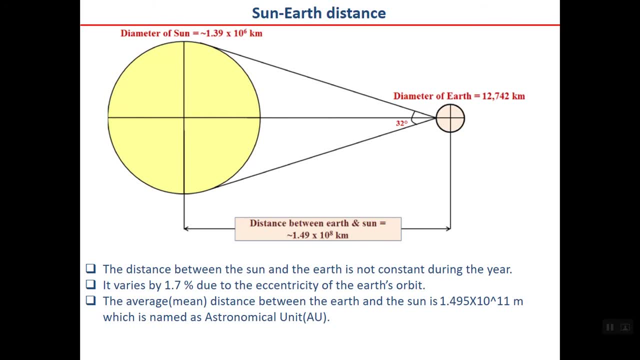 To have some exercise. Okay, let's start by the sun-earth distance. As you know or see in the picture, the diameter of the sun is much larger than the earth, And the distance between them is approximately 150 million kilometers. The important point here is that the distance between the sun and the earth is not the same. 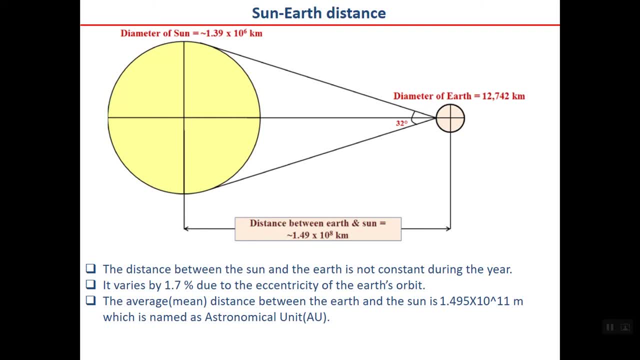 The distance between the sun and the earth is not constant during the year. It varies by 1.7% due to the eccentricity of the earth's orbit. So the orbit of the earth around the sun is not a circle. The average or mean distance between the earth and the sun is 149 million kilometers. 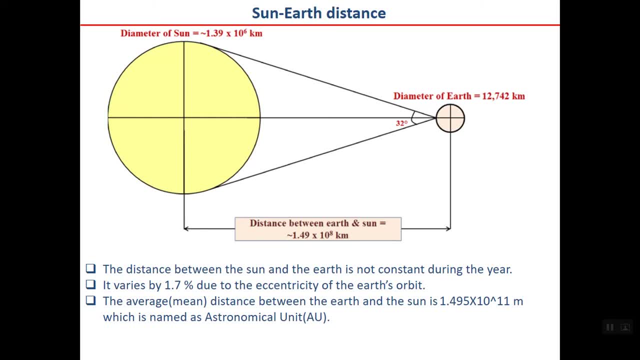 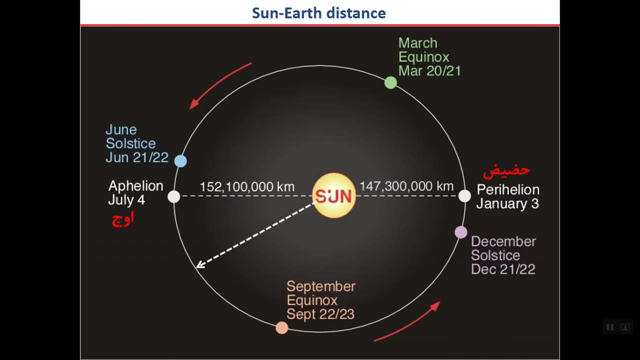 Which is named astronomical unit or AU. So further on, whenever you see AU, the meaning is astronomical unit, Which is around 149 million kilometers. The slide here shows the orbit of the earth around the sun. You can see that the minimum distance, which is 147 million kilometers, is on January, the 3rd. Which we name it Hazard, And the maximum distance is 152 million kilometers, Which occurs on 4th of July And the name is Ouj. So, unlike many other people may think, the minimum distance between the sun and the earth is not on summer. But it is in winter, And the same for the summer. You can see that in summer, actually in the middle of the summer, we have the maximum distance between the sun and the earth. So what is the reason for seasons? Actually, the reason for what we know as seasons is not the distance between the sun and the earth. 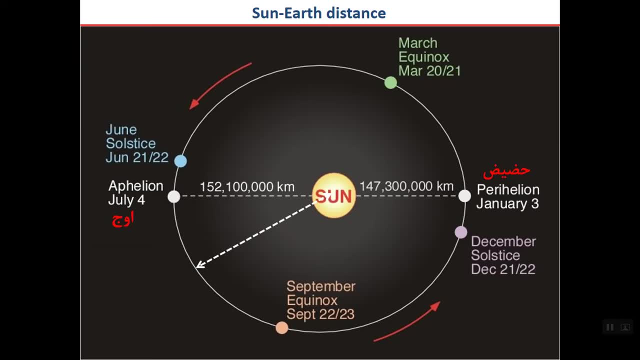 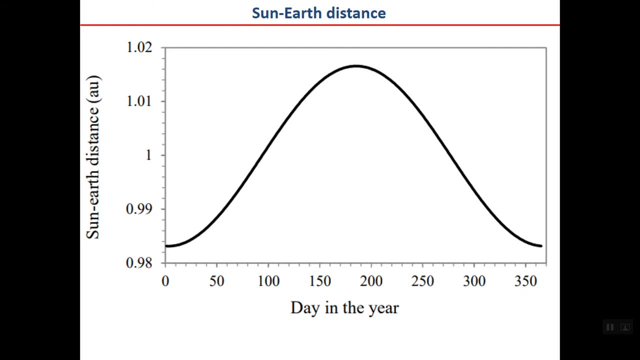 And actually the reason is another parameter, which is the declination angle, And we will discuss about that later. Here you can see the variation during the days of the year starting from 1st of January. You can see that the minimum distance is on January. 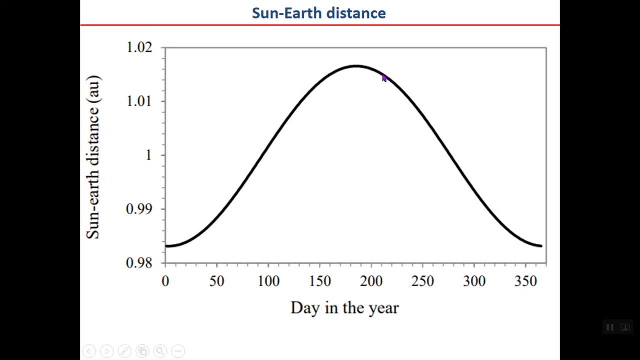 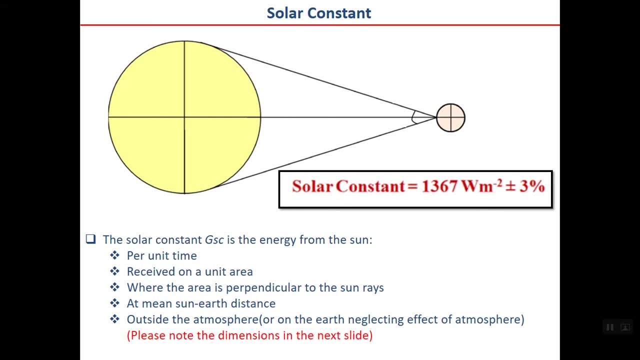 And the maximum distance, as you can see, is somewhere in the summer. The next very important parameter that we should learn is solar constant. Solar constant, as you can see here, which we show by G with the subscript SC, is the energy from the sun per unit time. 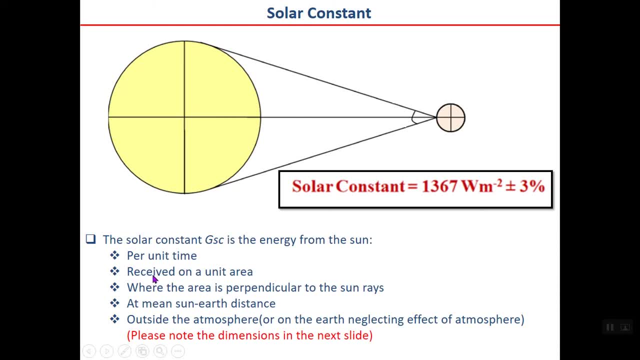 It means that it is joule per second, for example, Which is Watt Received on a unit area per square meter, And the area is perpendicular to the sun rays, Because you know that the angle of the surface with respect to the sun rays 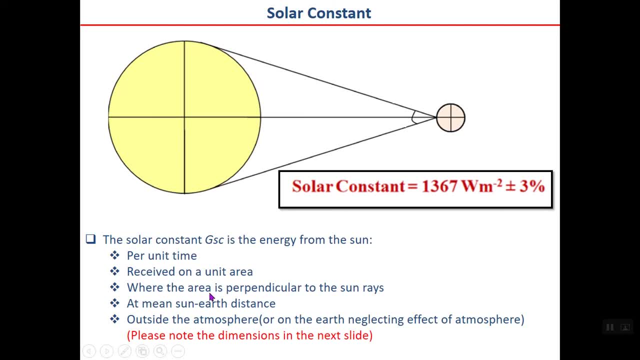 affect the intensity of solar radiation. So we are discussing about a plate which is placed completely normal to the sun rays And at mean sun-earth distance 149 million kilometers, And the important point is that outside the atmosphere or on the earth, neglecting the effect of atmosphere. 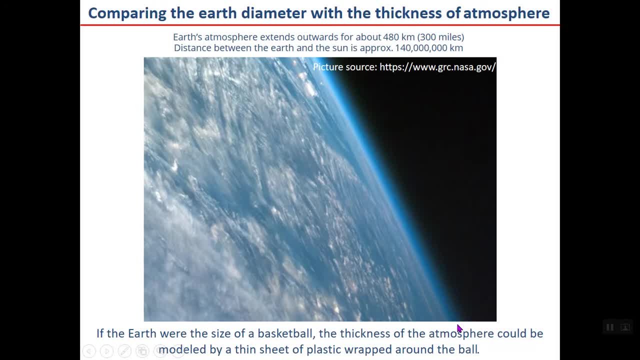 What's the meaning? See this picture, Which is a very interesting picture. Actually. the earth's atmosphere extends outward for about 500 kilometers, While the distance between the earth and the sun is 149.. Sorry, this is wrong: 149 kilometers. 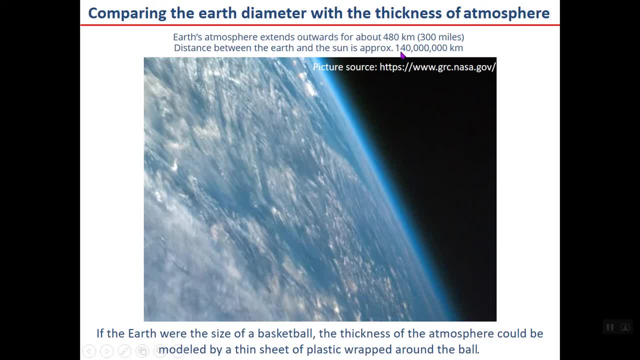 Or 150 kilometers if we want to round it. So you can see that the thickness of the atmosphere, as you can see here in this picture, And here you can see that if the earth were the size of a basketball, The thickness of the atmosphere could be modeled by a thin sheet of plastic wrapped around the ball. 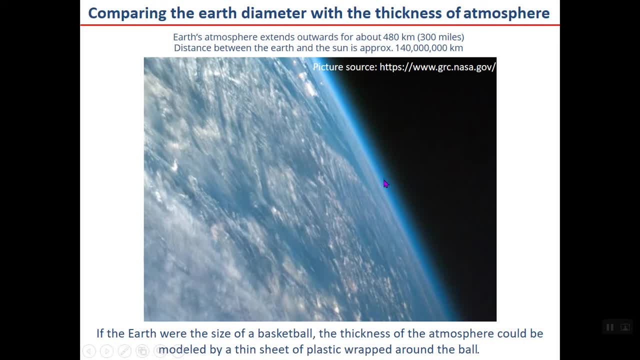 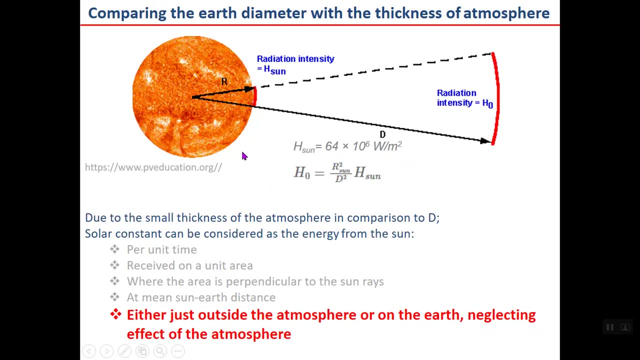 So the thickness of the atmosphere is very small, Both in comparison to the earth diameter and also in comparison to the distance between the earth and the sun. So whenever we discuss about the solar radiation, So the next, The other, The other important point is: 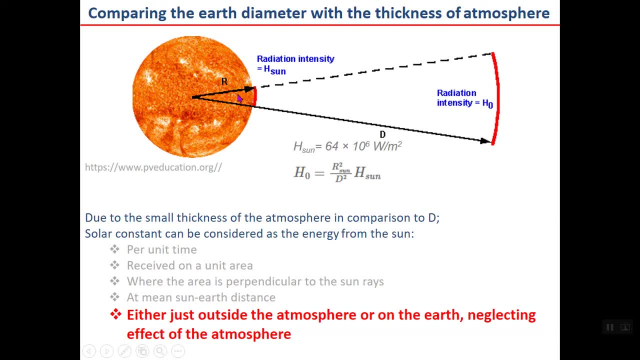 That, as you may remember from physics, The intensity of solar radiation. The intensity of solar radiation varies with the distance from the source of radiation. For example, if this is sun And the radiation intensity is h sun, Which is this value over the sun? 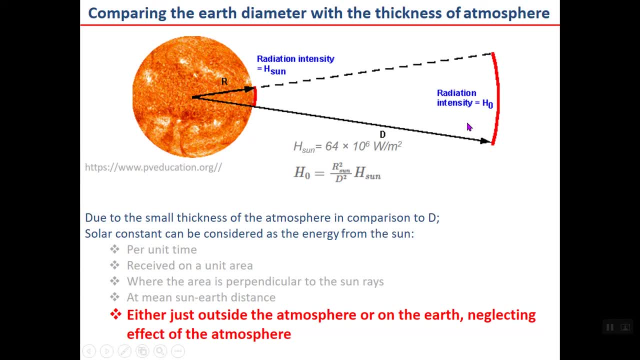 Then, when there's a distance between the sun and the earth, for example, Or any other planet, The intensity of the radiation on that planet, That surface, is proportional to d square reversed. So whenever the distance between the source of radiation and the receiving surface varies, 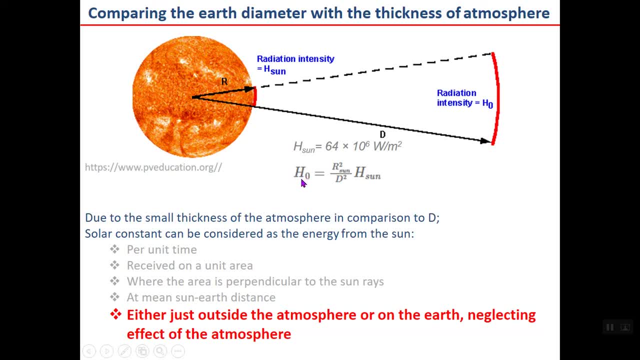 The intensity of radiation, as you can see here, also varies. So you can say that, due to the small thickness of the atmosphere in comparison to d Solar constant can be considered as the energy from the sun, As we told per unit time received, and even others. 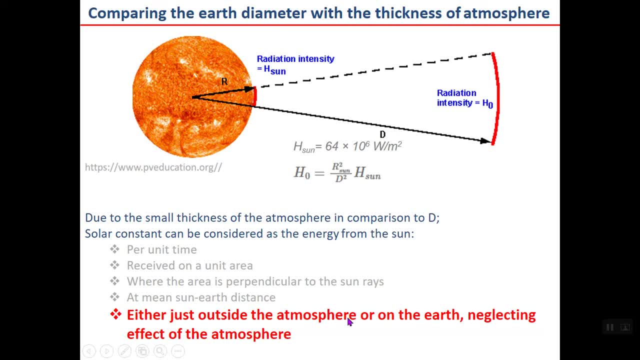 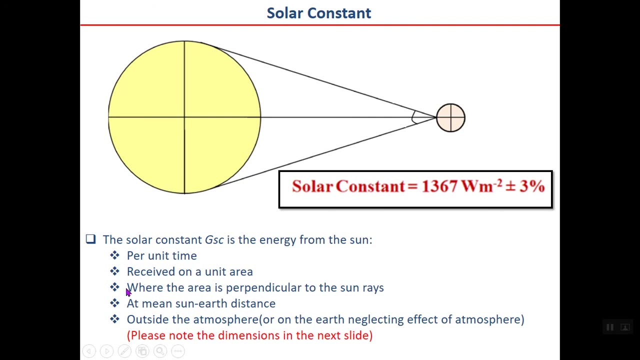 And either just outside the atmosphere Or on the earth, neglecting the effect of atmosphere. This means that you can say that Solar constant, as we told here, Is per unit time received and unit area Area is perpendicular to the sun rays At mean sun earth distance. 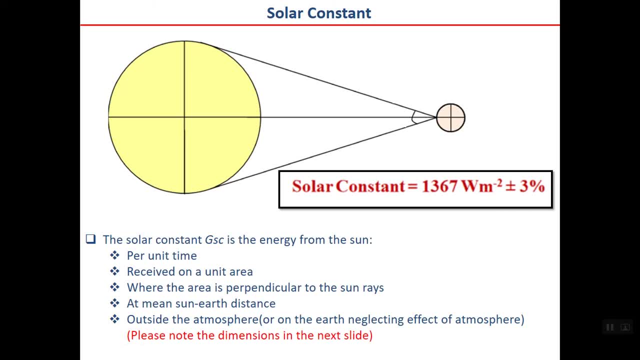 And where the plate or surface is installed, Either outside the atmosphere, Okay- Or on the earth, neglecting the effect of atmosphere. Actually, you know that atmospheric effect is very large on the solar radiation, But for the solar constant you can use either of these definitions. 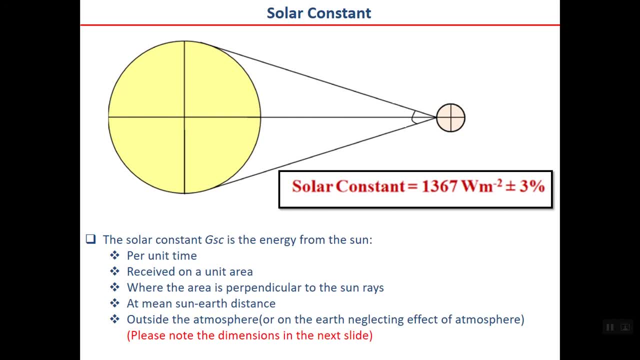 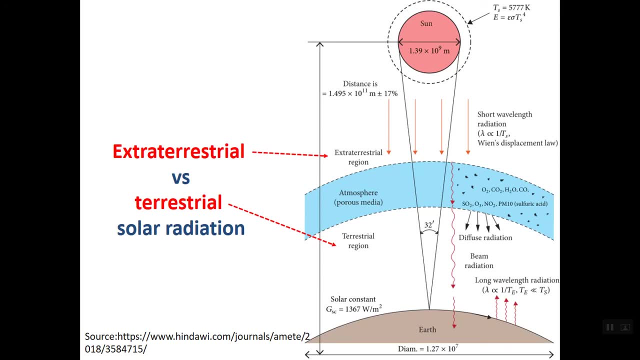 What's the value of solar constant? It's around 1367 watt per square meter. Become familiar with Here with two other definitions. You can see here the sun, The atmosphere And the earth. Actually, the atmosphere is extends to the earth. 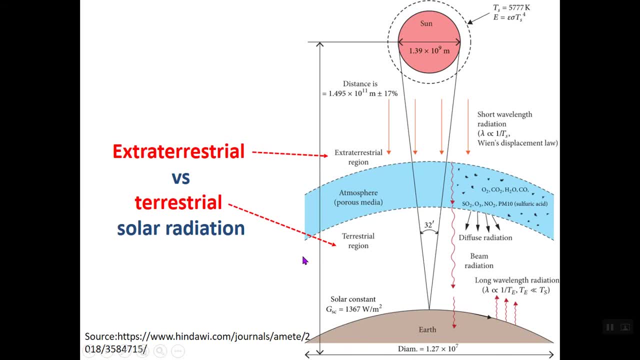 This figure may be somewhat corrected, But the solar radiation which is just outside the atmosphere boundary Here is named extraterrestrial radiation, And what we receive on the earth is terrestrial radiation. So whenever you see terrestrial and extraterrestrial radiation, The meaning is, as you can see, here: 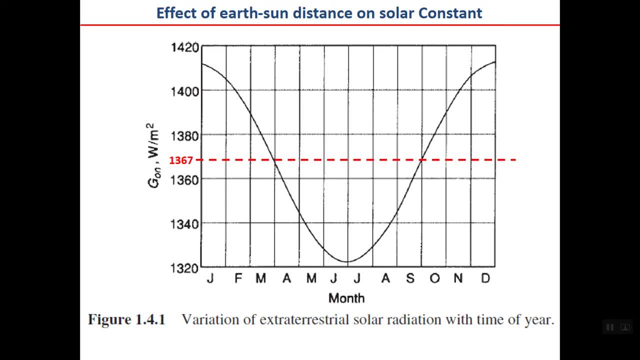 In this slide you can see the variation of solar constant During different months of the year. Here is January And you can see that solar constant has its maximum value. Why? Because the distance between the sun and the earth is minimum at this date. 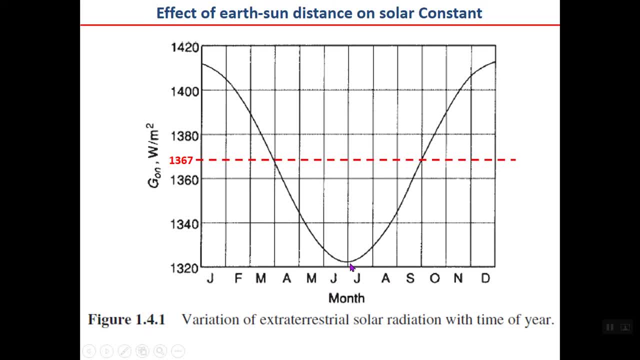 And here you can see that somewhere between June and October, Somewhere between June and July, in the summer, You have the minimum solar constant. Why It is so? because the distance between the sun and the earth is at its maximum At this time of the year. 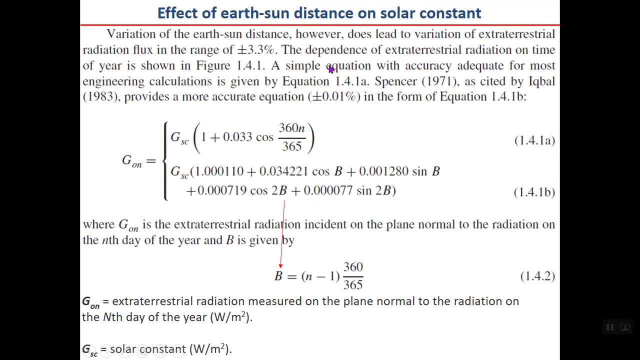 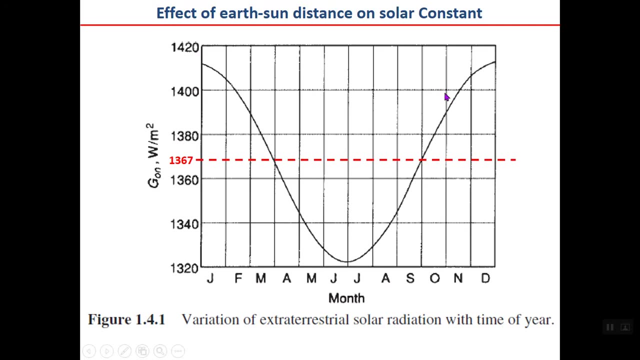 Okay, As the earth orbit around the sun is not a circle, So you can expect that the value of solar constant, As you can see in this slide, is not constant during the year. Is there any equation describing this curve? Yes, Actually, at least there are two equations in your book. 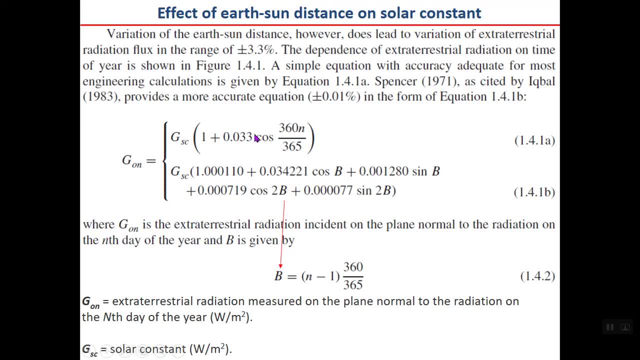 There are other equations, But these are enough for our course. The first is GON. You can see here that GON is extraterrestrial radiation Measured on the plane normal to the radiation on the nth day of the year. This is small n actually. 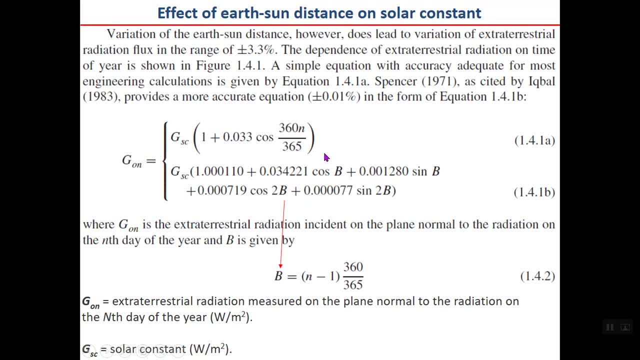 Which is shown by GSC. Multiplied by this parenthesis Here, n is the day number. By using this formula, Putting 1367 for GSC And n for the day number, You can calculate GON, Which is actually the curve shown in the previous slide. 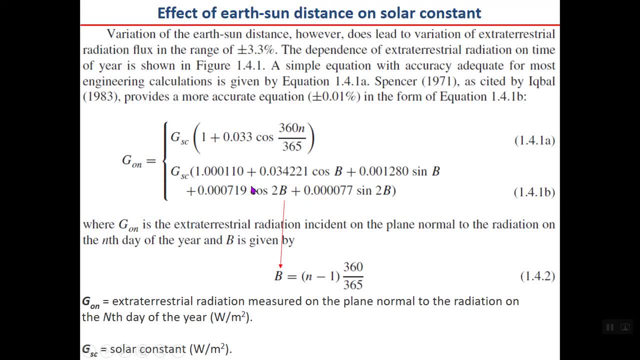 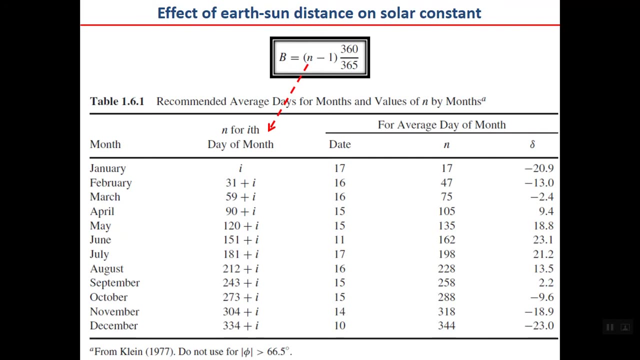 Either you can use this equation instead, Which is somewhat more complicated But more accurate. Here, b stands for the n-1.. Multiplied by 367.. Or 365.. How you can find n? Either you can calculate it yourself Or use this table. 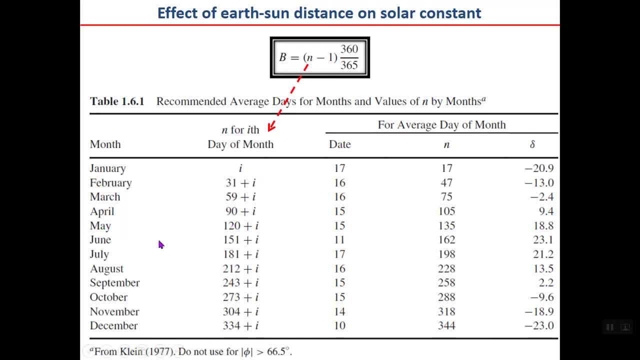 There is a table here. For example, if today is 10th of June, Then you will come to the row which shows June And then put 10 instead of. i. Adding 10 to 151 is 161.. Which is the day number. 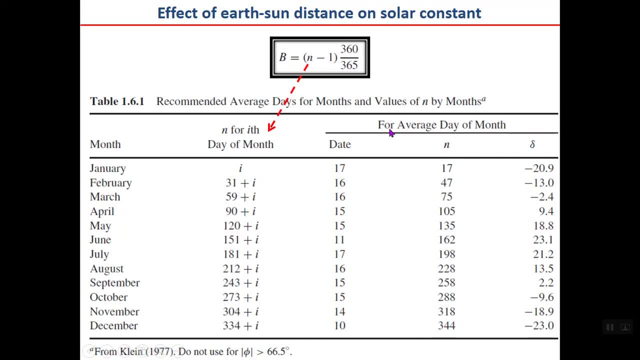 Here you can see other columns For the average day of the month. Actually, we have an average day for each month. It is not actually the middle of the month, as you can see. It is based on the solar radiation averaging And for each month. 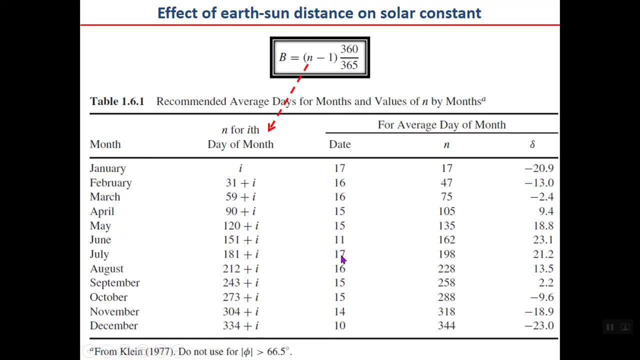 For example, for the month of July, 17th of July is the average day of the month And what is the day number? Exactly by the same formula shown here You can calculate the n And this is the declination angle Which we will discuss about that later. 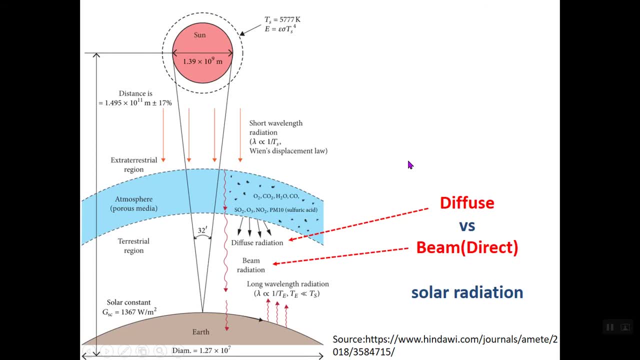 The next definition is the definition of diffuse And beam or direct solar radiation. We told before that Sun rays passing the empty atmosphere, Which is the extraterrestrial region, Comes to the atmosphere And then Its either its spectral values Or its intensity will be varied. 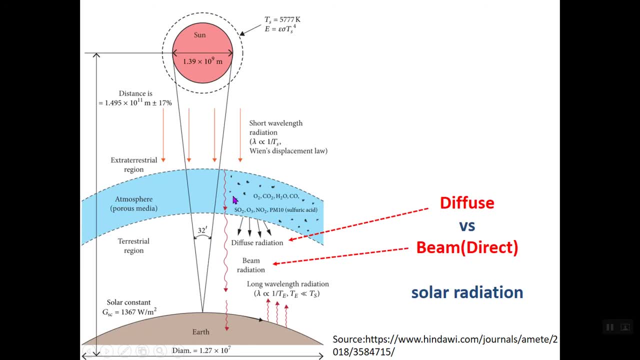 By the molecules And maybe other Matters that are Substances that are in the atmosphere, For example, Like the one you can see here. The most important definition here Is dividing the total solar radiation Coming to the earth Into diffuse and beam radiation. 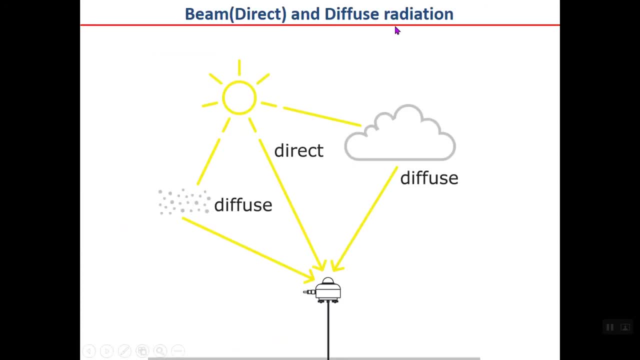 As you can see, This picture may show it better. Direct solar radiation Is the radiation which Comes directly from the sun rays Without scattering. For example, This may be either a solar sensor Or a solar collector Or solar photovoltaic module. 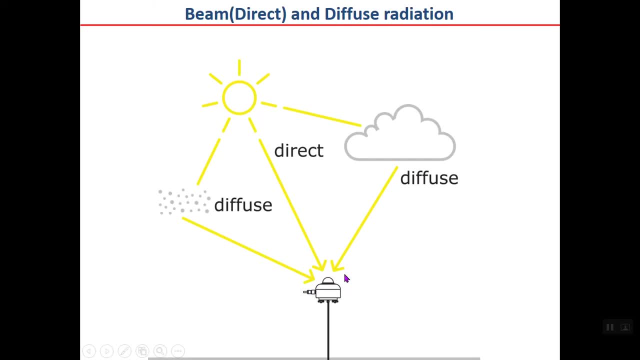 Or any other Desired element or surface, But The solar radiation Which hits to, for example, Clothes or other particles Which are existing in the air, Like dust, Like other molecules in the air, Pollution or something like this, And then again, 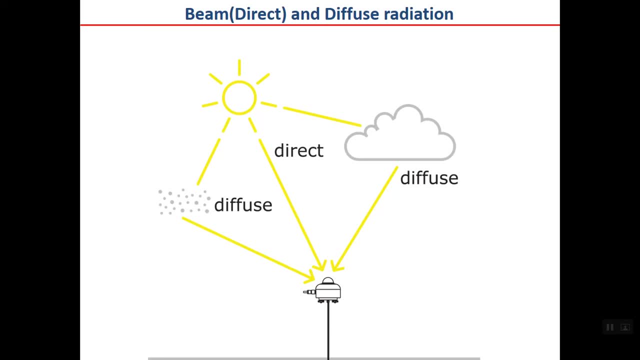 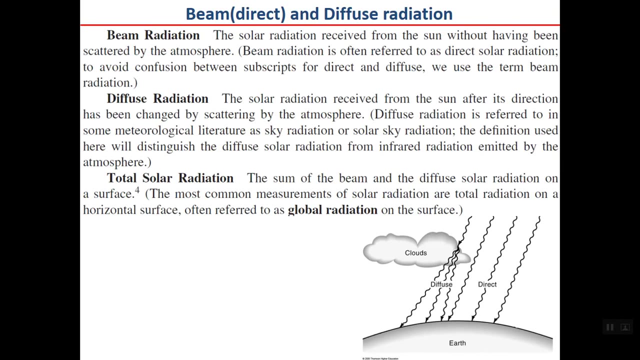 Comes to your surface. Your desired surface Is then diffuse solar radiation. So we have either direct Or beam solar radiation And diffuse solar radiation. Here you can see the definition Which shows better the meaning. Beam radiation is the solar radiation. 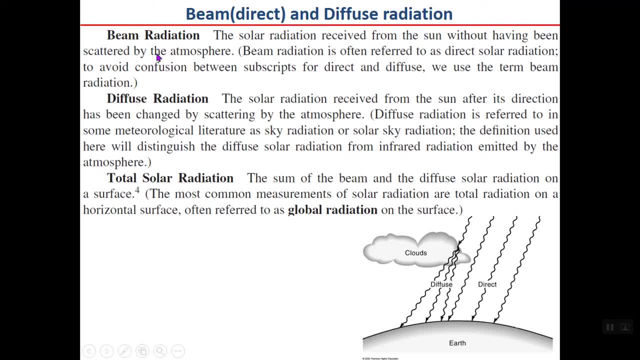 Received from the sun Without having been scattered By the atmosphere, And generally in this book Or in this course, We use beam radiation Instead of direct solar radiation To avoid confusion Between subscript for direct and diffuse, Because you can see that. 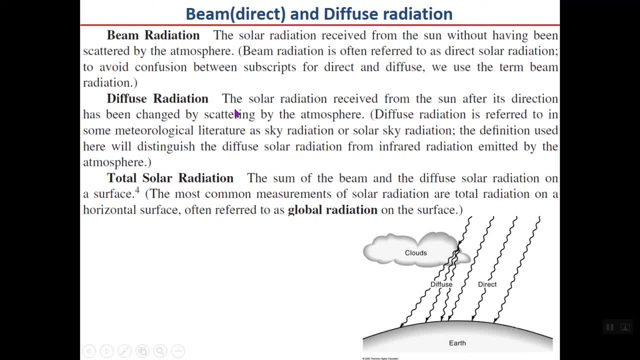 Both start with D. What is diffuse radiation? Diffuse radiation is the solar radiation Received from the sun After its direction has been changed By scattering by the atmosphere Or anything which is Existing in the atmosphere, And the sum of these two radiation. 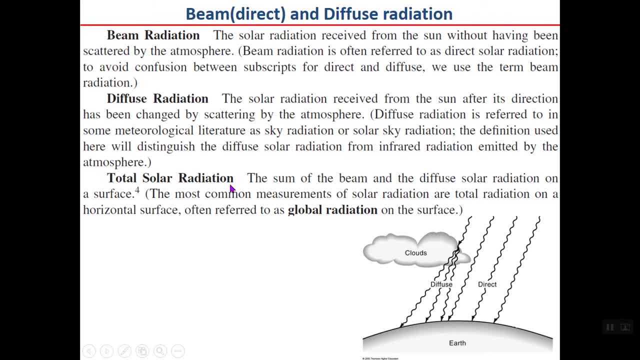 Beam and diffuse radiation Is the total solar radiation, The sum of beam and diffuse solar radiation On a surface- And the most common measurement Of solar radiation Is on a horizontal surface- And the total solar radiation On a horizontal surface. 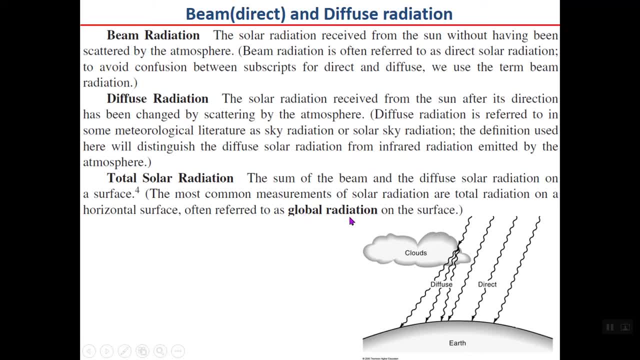 Is then global radiation, Or global horizontal irradiation, To emphasize on the fact That this is on a horizontal surface. So whenever you see Global horizontal irradiation Or total solar radiation, It is the sum of beam and diffuse solar radiation. 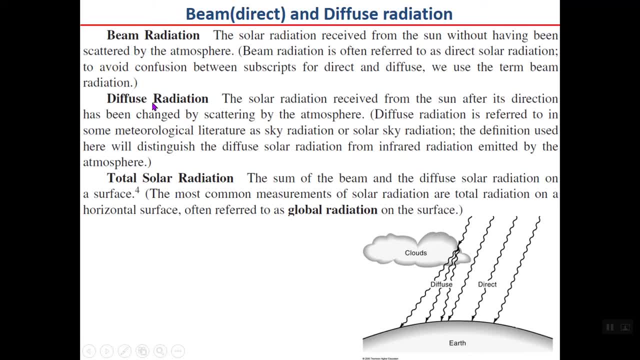 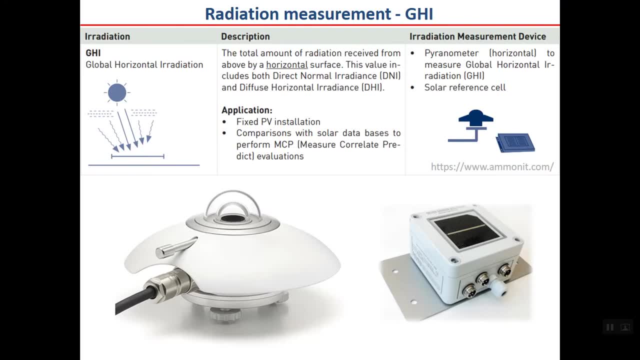 On a horizontal surface, How you can measure The solar radiation. This is a very complete topic That we will not cover in detail. Actually, I just want to show you How the solar radiation Is measured And how you can measure. 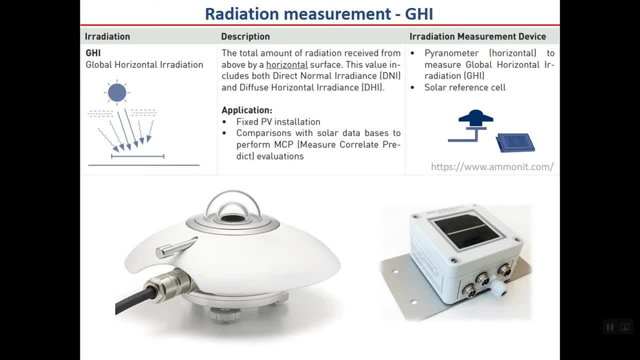 The total solar radiation On a horizontal surface Is measured Just in some simple, With some simple slides. Okay, The first is GHI. As I discussed, I told you just now In the previous slide, GHI stands for global horizontal irradiation. 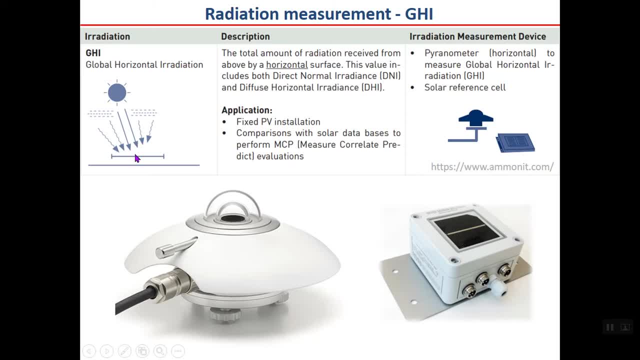 It is the total solar radiation On a horizontal surface. What is the irradiation? Because you can see That this is a new parameter here. We will discuss about that. Just I want to emphasize that It is the energy, You know. 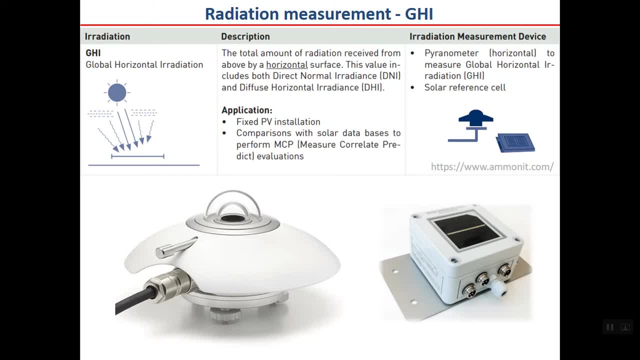 Because we have two types of solar radiation: Solar radiation intensity, Which is instantaneous, Exactly at this time, And solar energy, Which is the summation of solar intensity Or irradiance During, for example, a day. This is the solar energy. 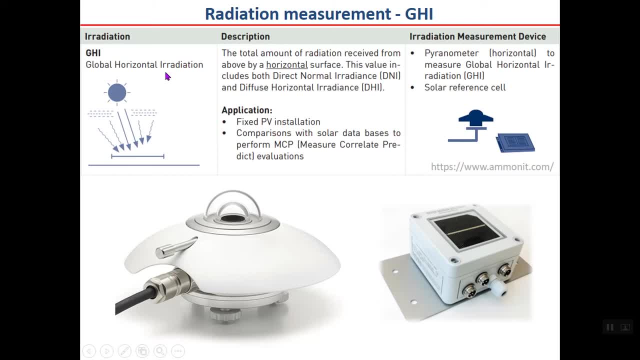 Not the intensity, It is not power, It is energy. GHI is global horizontal irradiation. So What is this? The total amount of radiation Received from above. Above means above the surface, By horizontal surface. This value includes both direct and diffuse. 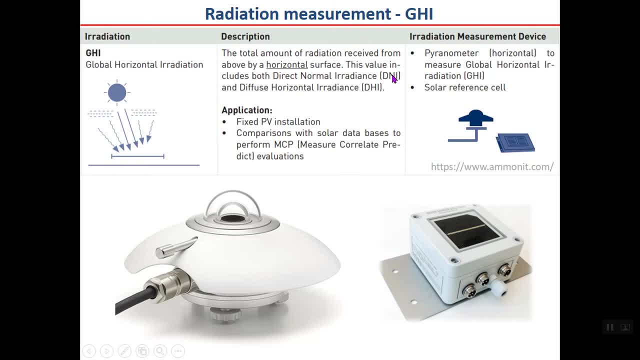 Horizontal irradiance. For the direct, You can see a new parameter, DNI, And for the diffuse, You can see a new parameter, DHI, Which is the radiation Metrological stations And also in solar power plants, How it can be measured. 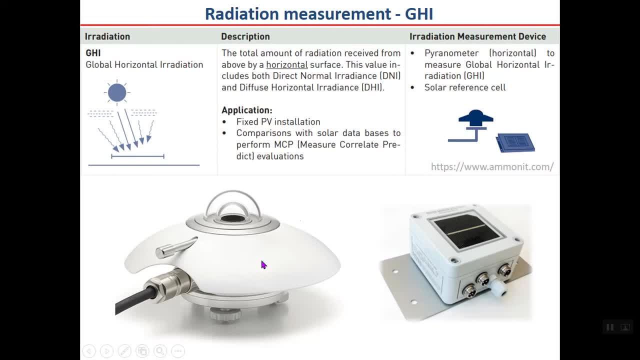 There are generally two methods. The first is a pyranometer. You can see here A horizontal pyranometer To measure global horizontal irradiation. There is a sensor, Generally here In the black area, You can see it. It is a thermopile. 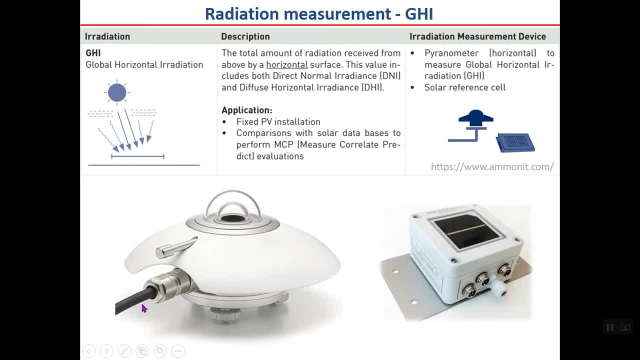 And there is a glass dome And the signal is produced Where the signal is proportional To the intensity of solar radiation. There are also Other sensors Which are named solar reference cells. These are actually a simple Solar cell, as you can see. 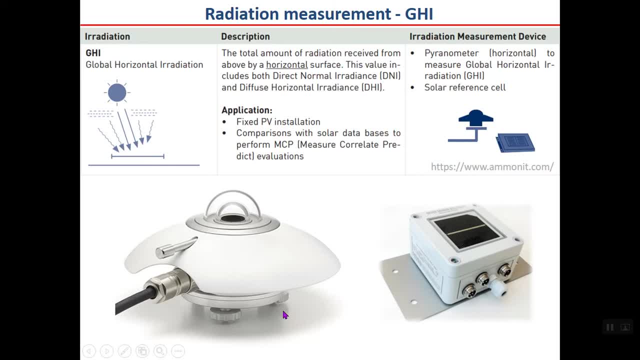 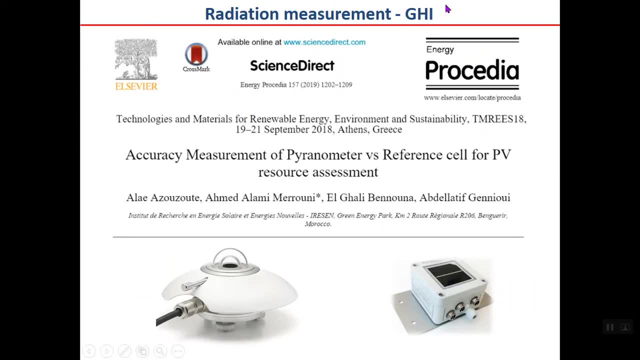 There are differences between the two, But in general This is much more accurate, Especially for research works. But if you want To know more about the differences Between the pyranometer And reference cell, There is a good paper You can see here. 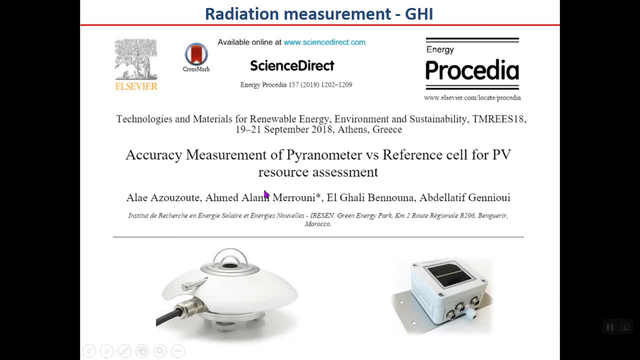 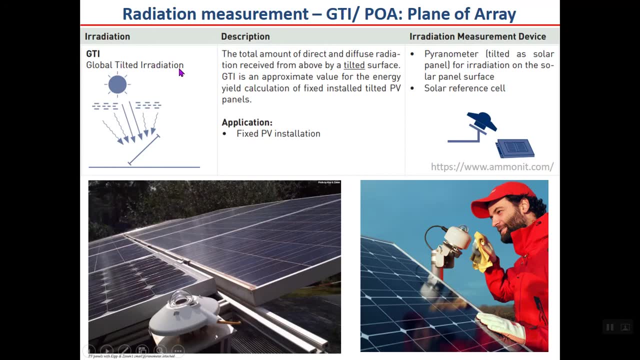 The topic is accuracy measurement Of pyranometer versus reference cell For PV resource assessment. The next measurement Is GTI, Which is global tilted irradiation. As you can see, It is the total amount Of direct and diffused radiation. 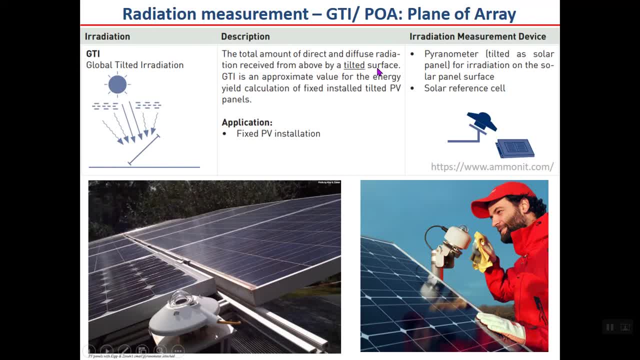 Again like the previous one, But received by a tilted surface- Tilted surface, The one you can see here, Which are tilted, Because you know that generally, Or in most cases, Solar modules or solar collectors Are installed at an angle. 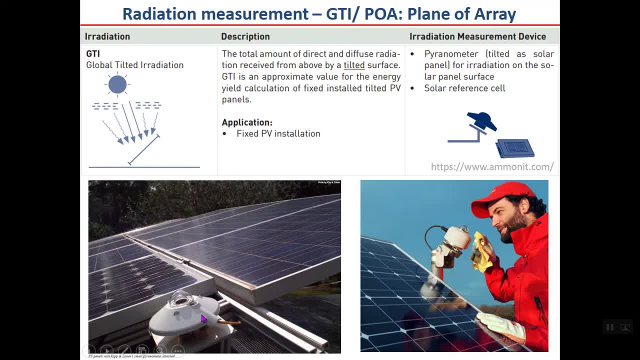 Or tilted. So if you measure the solar radiation On the tilted surface, Which is certainly different With the radiation on horizontal surface, This is named GTI. I want just to emphasize once again That the angle of the surface And the radiation intensity 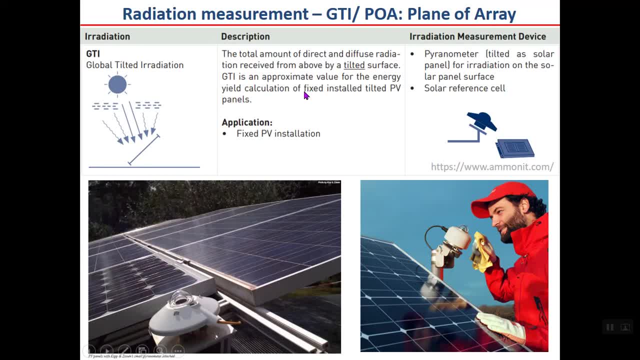 We will discuss about that later. GTI is an approximate value For the energy yield calculation Or fixed installed tilted PV panels. What is the meaning of yield? Yield is what you You take from the sun By the PV modules, By installing a pyranometer. 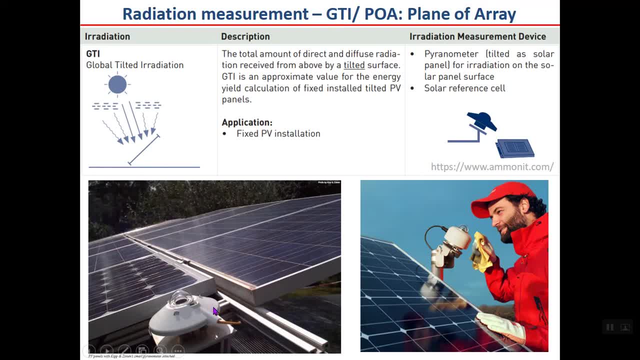 In a tilted array, Tilted plane- actually, You can estimate How much energy Your panels should produce And then you can compare With the actual results. As you can see, This is the application, How it is measured: Just by tilting the pyranometer. 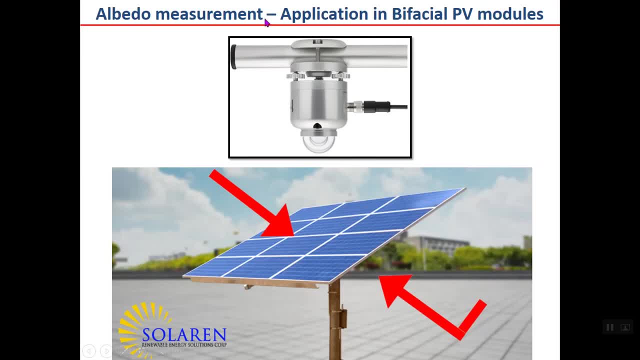 Or the reference cell. Another measurement Is the Albedo measurement. Actually, there is a new application. Albedo measurement Has a lot of applications In agriculture Or in metrological stations, But there is a new application Which is called. 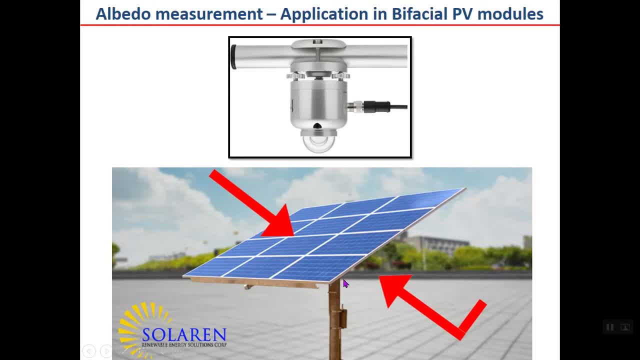 Bifacial Solar Modules. Bifacial- Bifacial means two-phase. These are modules Because generally in common PV modules You will receive sun from above And the panel produces power, But in the bifacial modules The backside of the module, 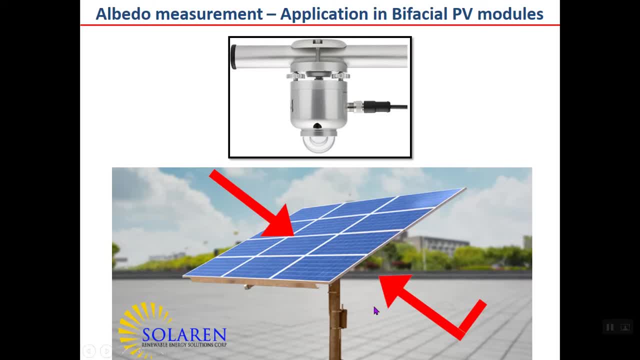 Also can receive light And produce energy. These are named bifacial modules. For this type of modules It is important to know Albedo. So this is a device Which is used for measuring albedo. For accurate measurement There are some more complications. 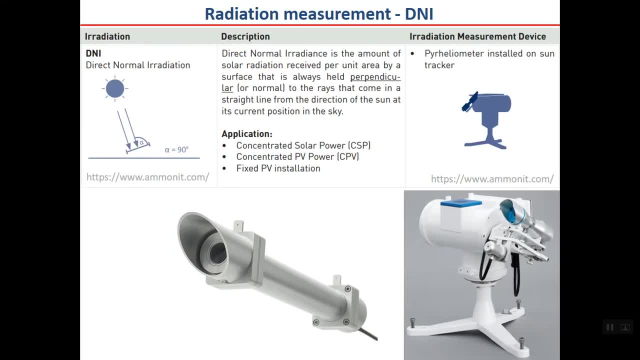 And sophisticated calculations Needed, which are outside The scope of this course. The next parameter Is DNI. DNI is direct normal irradiation. Direct normal irradiation: As you can see, Direct normal irradiance Is the amount of solar radiation. 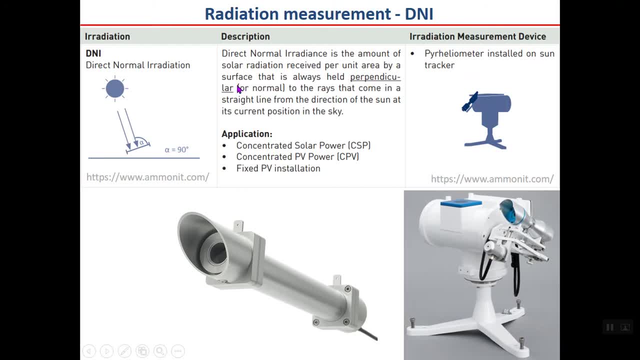 Per unit area By a surface That is always perpendicular Or normal to the rays. This is very important. So if you have a sensor Like the one you can see here, The sensor is at the end here And there is a hole. 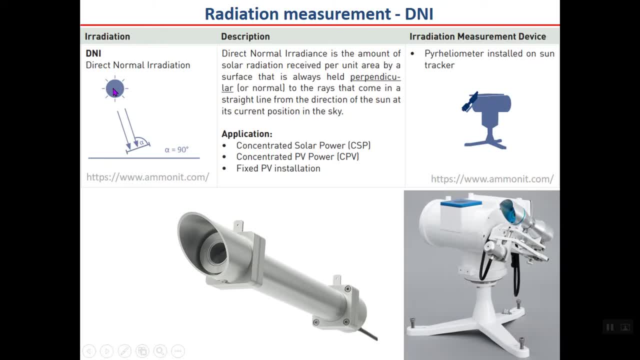 There is a long hole In this tube If you direct this sensor to the sun, Like the one you can see here, And then it will measure DNI Or direct normal irradiance By a device named Per heliometer. 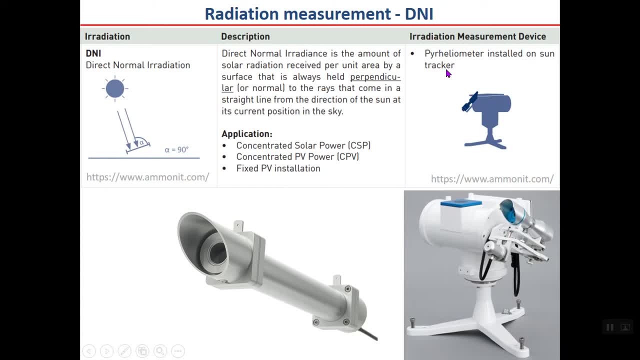 But installed on a sun tracker. What is sun tracker? Sun tracker is a device that tracks or follows the sun, Because the position of the sun In the sky is not constant During the day, Why a sun tracker Or solar tracker is needed. 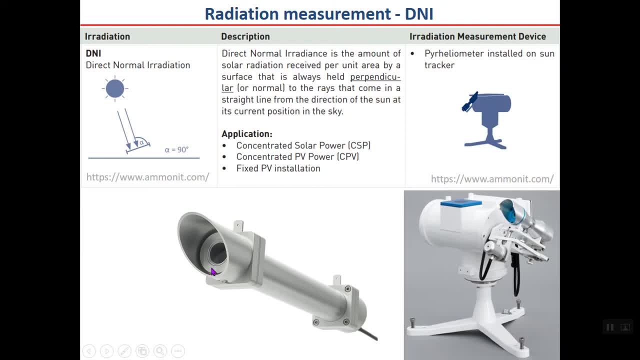 Because the position of the sun is not constant And if you want to direct- To always direct- this sensor Or this tube Towards the sun, You should move this sensor. So a solar tracker is required, Like the one you can see here. 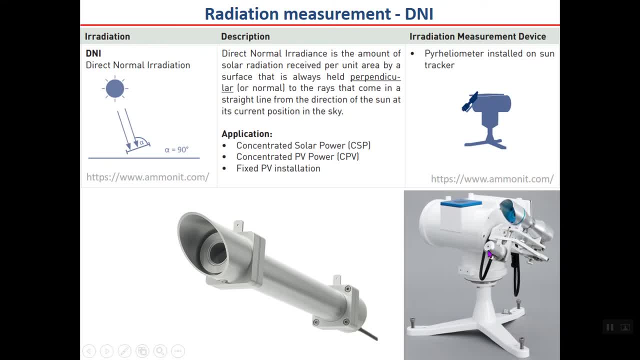 This stand is a fixed stand, And then the device, as you can see, Can rotate either horizontally Around the vertical line, Like the one you can see here, Or it can have an angle, And this is the sensor. So by always. 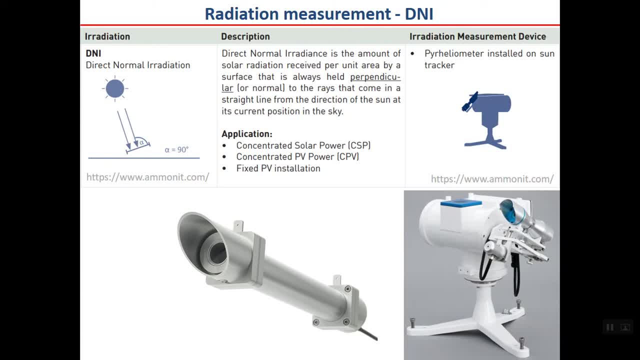 Putting the device Or sensor In such a manner That it is directed towards the sun. Then you can measure Direct solar radiation, Or DNI. Please note that By measuring direct normal irradiation, Like the one I told here, 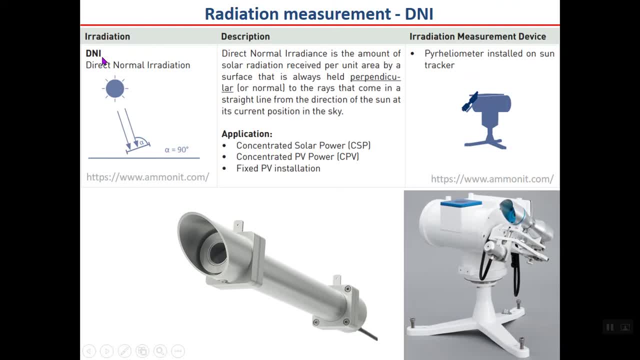 Then the sum of DNI And diffuse solar radiation Is not equal to the total solar radiation. We will discuss about that later And these are the applications. As you can see, You may know Or will learn later- Solar surfaces may be either. 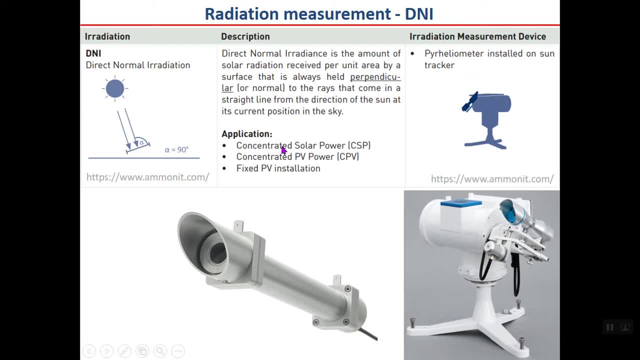 Non-concentrating Or concentrating In the concentrating part. We have concentrating solar collectors And concentrating photovoltaics And generally Concentrating collectors Are used to produce solar power, And concentrating PV Can also be used To produce power. 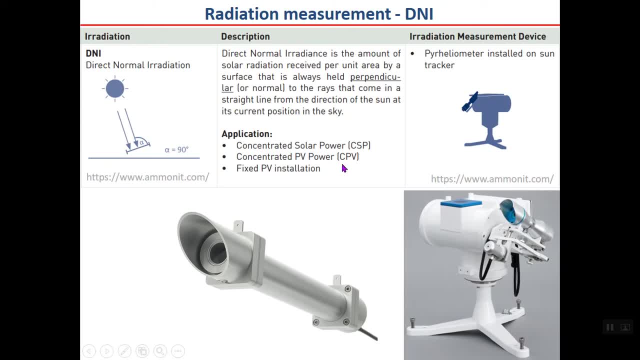 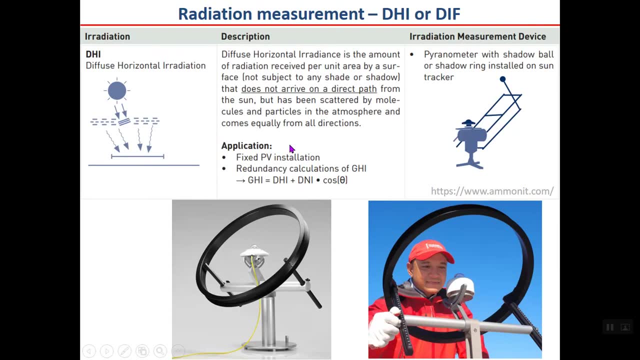 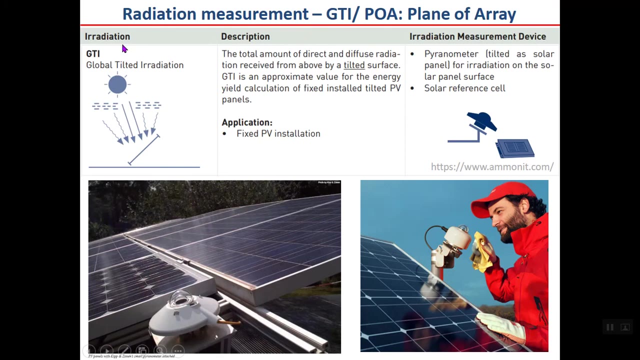 We will discuss about this later. The first is named CSP-CPV, And why? Why is it important for these types of devices? I will explain Within the next slides, The next: I forgot to say something Here, I think. 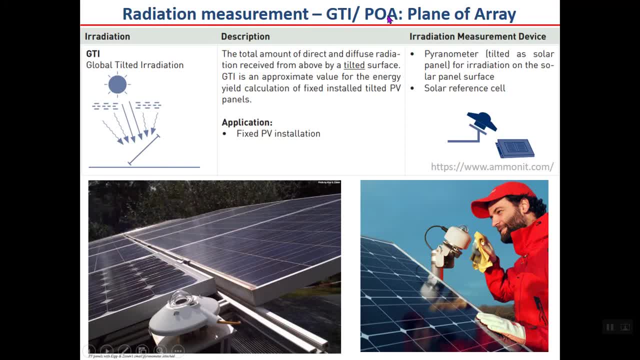 GTI or global tilted area irradiation. Sometimes you may see POA. POA is plane of array. Array means Array of modules And if the sensor Is installed in the same angle As the arrays, Then we can say: 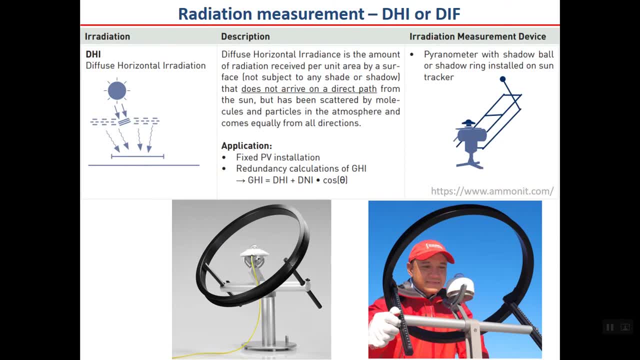 POA, or plane of array. Okay, The next solar radiation measurement Is DHI, Or diffuse horizontal irradiation. Diffuse horizontal irradiation Is the amount of radiation Received per unit area By surface Not subject to any shade or shadow. 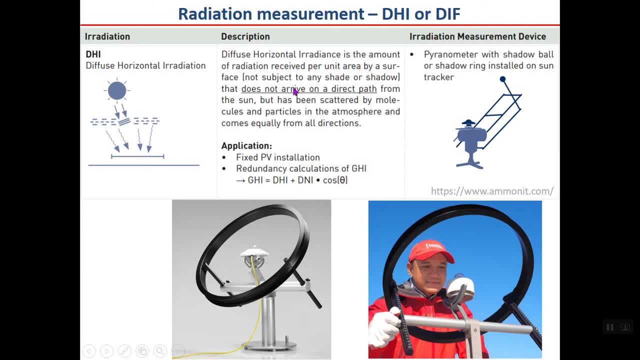 That does not arrive On a direct path from the sun, So in some way You will prevent the direct sun rays To hit the sensor. How it is measured? It is measured By the same pyranometer, As I explained before. 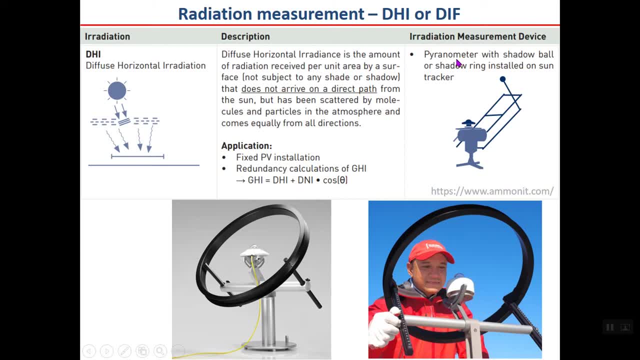 In the previous slides. But But with a shadow ball Or shadow ring. You can either have a shadow ball Like the one you can see here- This is a shadow ball- Or a shadow ring Like the ones you can see here. 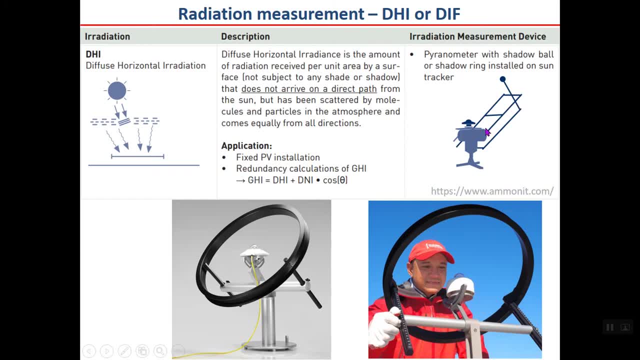 Generally, if a shadow ball Is used, Then you need a solar tracker also, Because the ball Should always put a shadow On the pyranometer Shadow of the sun. Okay, But if a ring is used Like the one you can see here, 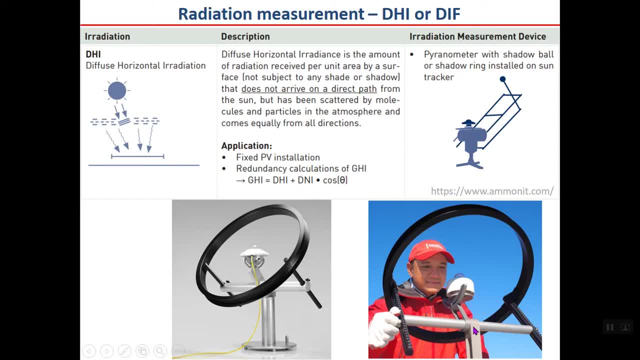 You generally can adjust the ring Manually, For example per week, Because the angle of the sun Or the path of the sun Will be different. It is not required To change the position each day, But it is good to change. 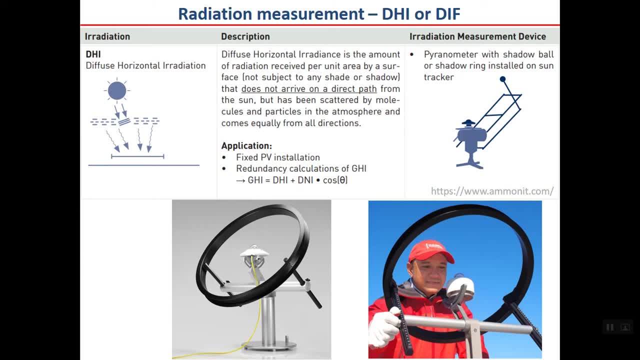 The position of the ring, For example, per week We may find time To discuss about this topic, Which is also very important Later, As I told you just now In the previous slide. The application is for fixed PV installation And the calculation of GHI. 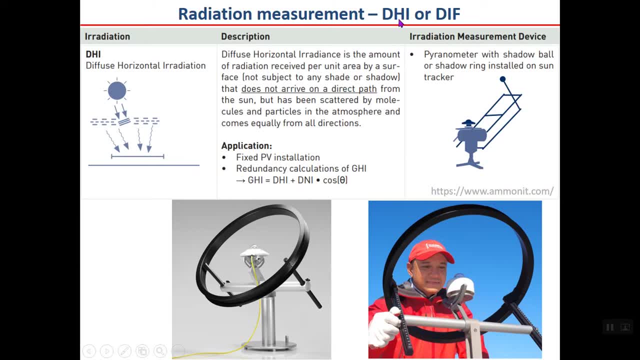 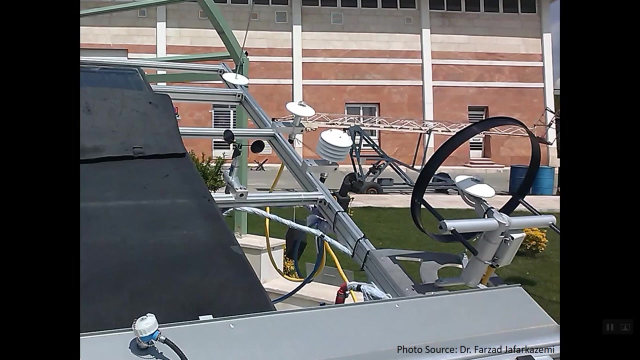 Can be done Also in this way, The, But just remember That there is such a formula. You can see here A Solar Diffuse, solar radiation Measurement device. As you can see here, This is a test lab Manufactured by me. 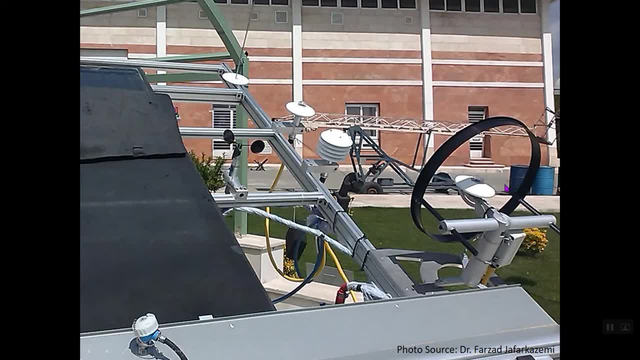 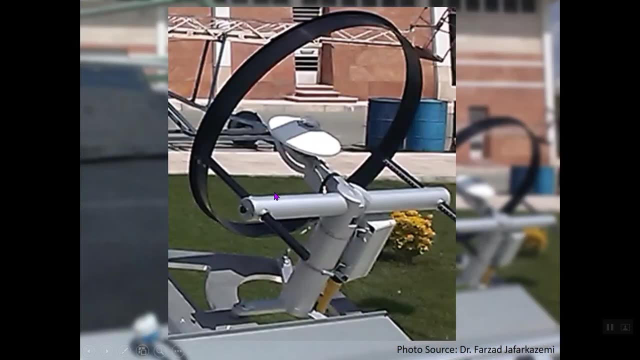 And it is used for testing solar collectors. We also measure The different parts of radiation. For example, here We have a pyranometer, Here we have air temperature measurement. This is the wind velocity measurement And this is the Sensor for. 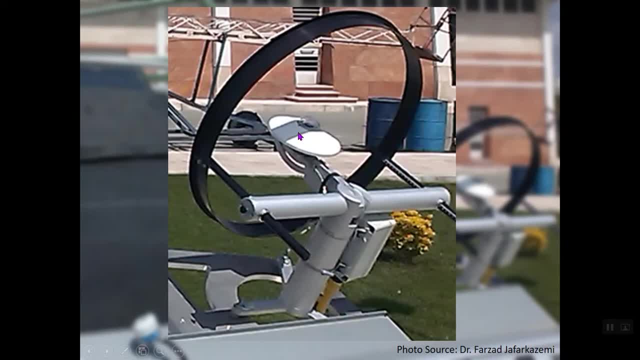 Measuring the Diffuse solar radiation. As you can see, There is a shadow on the pyranometer Which is produced by this ring. You can see, And per week- Once a week- We adjust the ring position And angle. 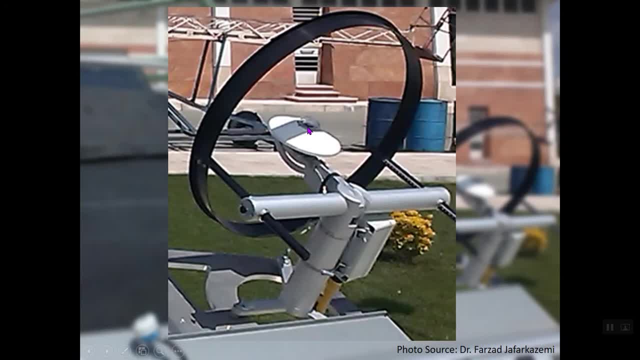 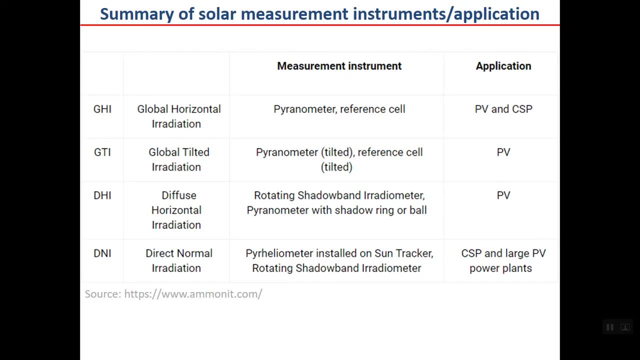 Because it should put A shadow on the sensor From sunrise to sunset Each day Within a year. Okay, There were four main. There were more, But these are the main. one, GHI, Which is global horizontal irradiation. 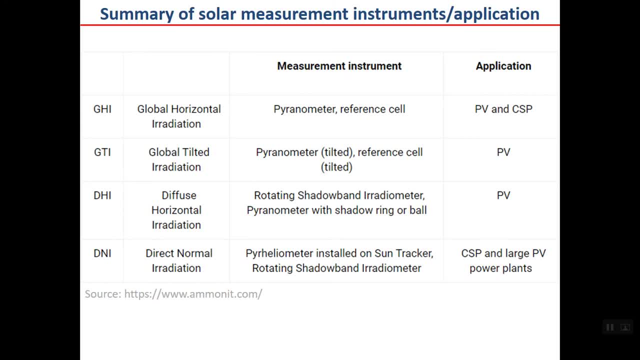 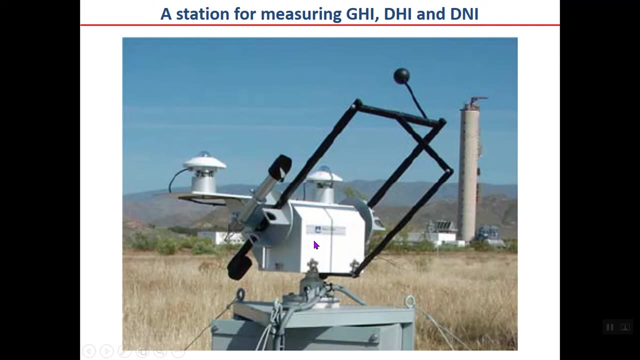 GTI, Which is the same on tilted surface, DHI or diff, Which is diffuse horizontal irradiation, And DNI, Which is the direct normal irradiation. Here you can see The measurement instrument And the application in summary, And also here you can see: 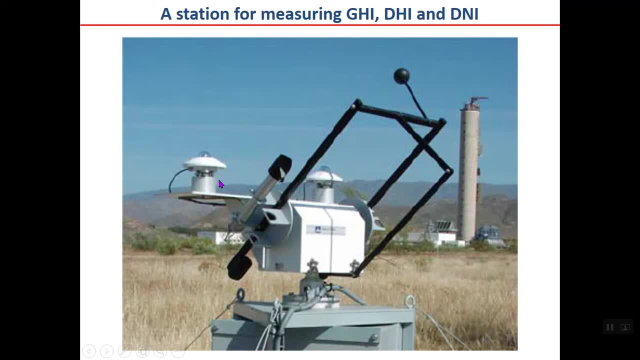 What is this? Just think a moment. Yes, this is a pyranometer For measuring horizontal irradiation. What is this one? Yes, this is a pyranometer With a shadow ball, As you can see here, Which is installed on a solar tracker. 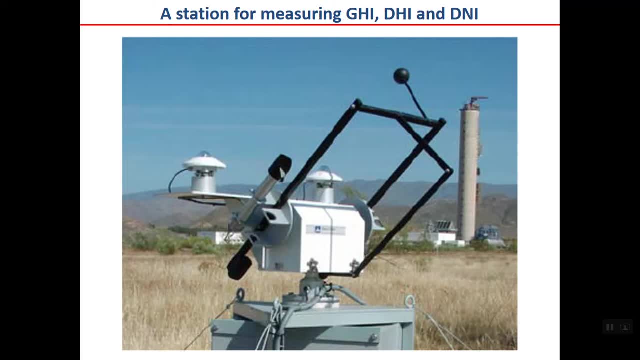 To put a shadow on the sensor, And so it measures The diffuse horizontal irradiation, Or diff. And what is this? Yes, This is a pyranometer Which measures Direct normal irradiation, Or DNI, And, as you can see, 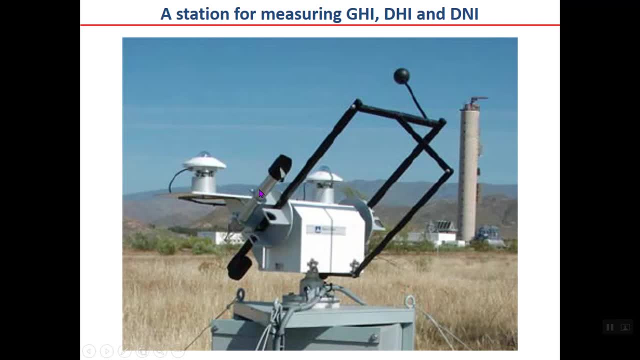 It is also installed on a solar tracker device, Because it should always Track the sun And direct toward the sun. Okay, For this there is no difference, Because when you rotate the device, This sensor always Is held in a horizontal position. 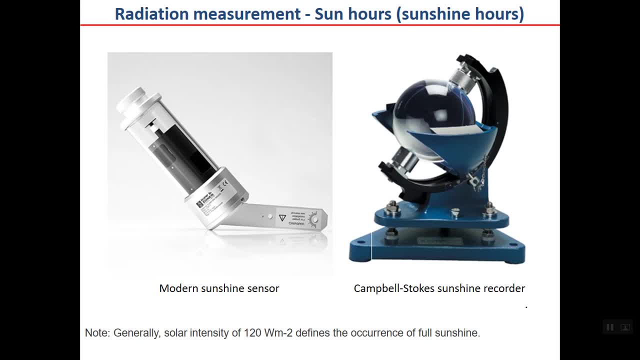 So always it measures Horizontal irradiation. Another measurement parameter Which is important And generally used in metrological stations Is sunshine hours Or sun hours. Actually, the sun hours, As you can see here, Is the hours when the sun shines. 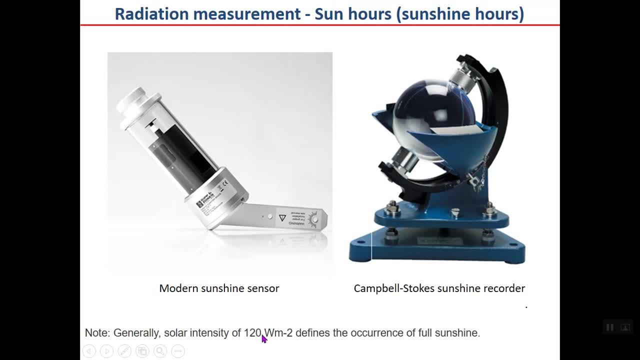 With an intensity of more than Equal to more than 120 watt per square meter. So if, During a day Which may be, for example, 6 hours, For example, You have 6 hours of sunshine With an intensity more than. 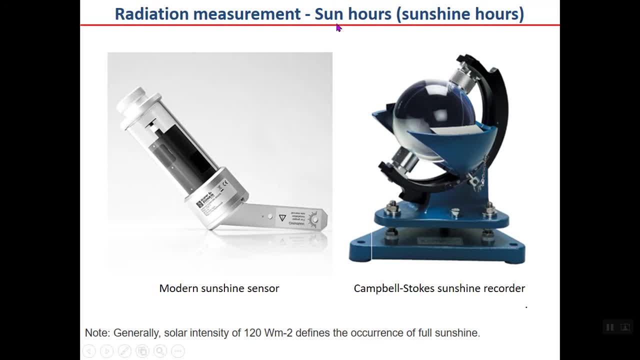 120 watt per square meter, Then 6 is the Sunshine hours Or sun hours a day. We will use this parameter In our calculation later. It may be Measured by old instruments Like the Campbell Stokes Sunshine recorder. 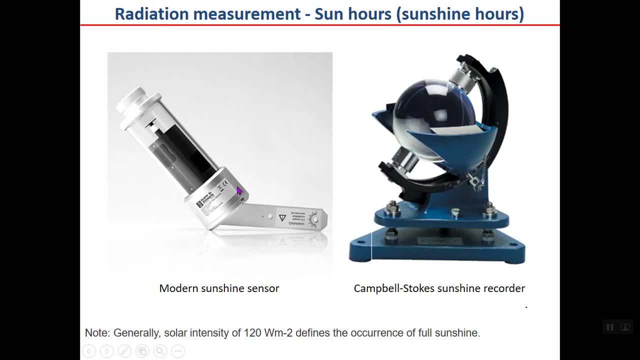 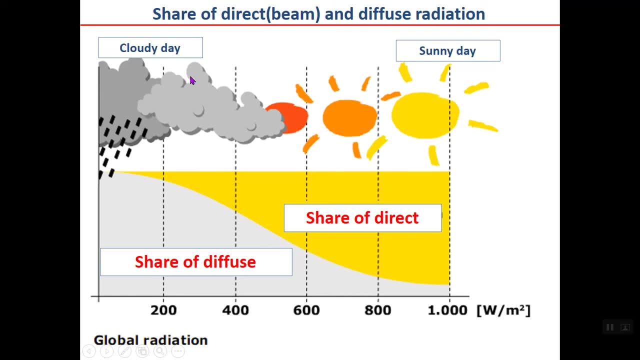 Which is an old instrument, Like the one you can see here, Which are more common in these days. The graph here Shows an interesting, Interesting Curve Which shows the Share of direct and diffuse solar radiation. You may ask Yourself, for example: 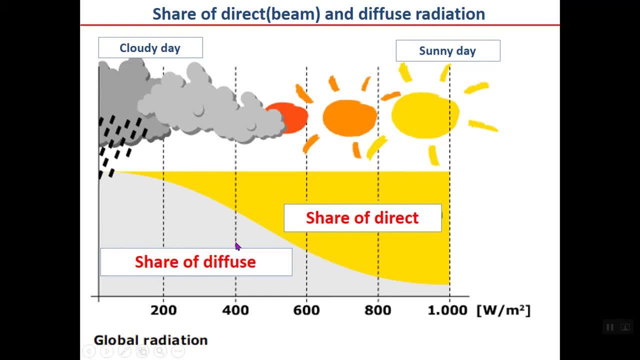 Just know What is the share of Diffuse and direct solar radiation Outside? Actually, the Diffuse solar radiation Depends on the Climatic condition. If it's a completely sunny day, Let's start from here. It's a completely cloudy day. 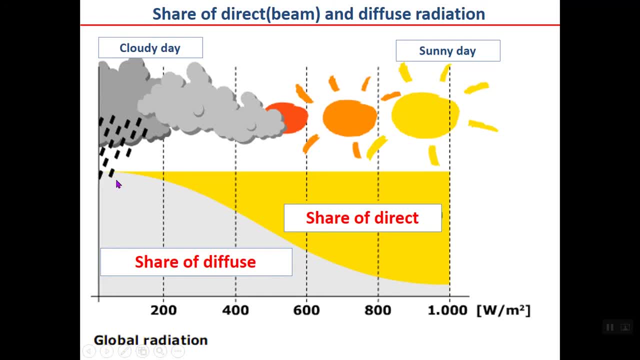 Then 100% of the Solar radiation is Diffuse solar radiation, Because when it is completely cloudy There is no sun rays at all. So the direct radiation, Or beam radiation, is zero And 100% is Diffuse radiation. 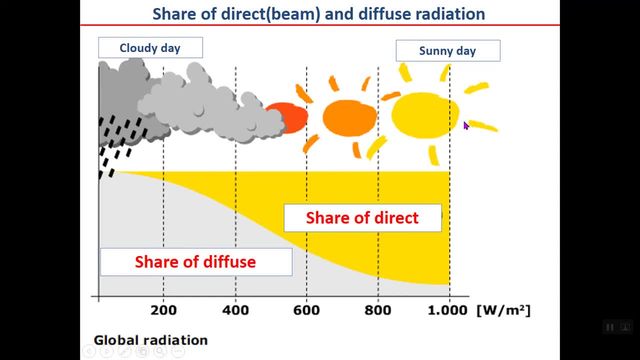 If you go to the More sunny condition Or a completely sunny day, Then you can see that Most of the radiation is Direct solar radiation. You may be surprised Why it is not 100% Like the one you had here. 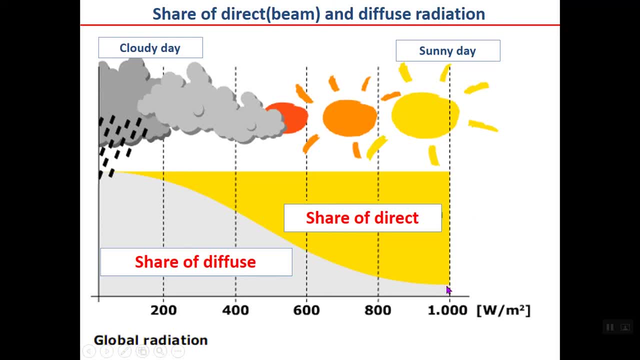 Because even in a completely sunny day, There may be some molecules in the air Or dust Or something like this. You can see no cloud, But there are other particles, dust or other things That may scatter the sun rays. So even in a cloudy day, 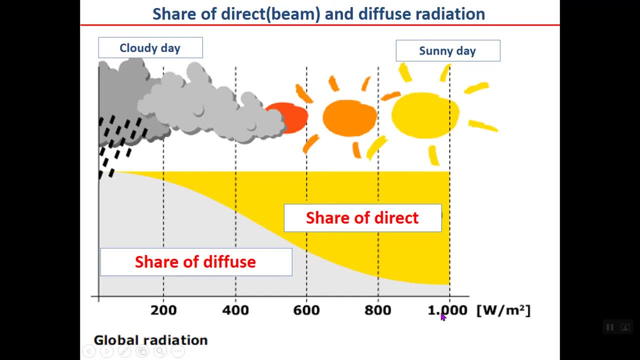 For example, If the total, for example, Solar irradiance May be 1000 watt per square meter, Then Then, For example, 100 watt per square meter May be diffuse And 900 may be direct solar radiation. Just one point. 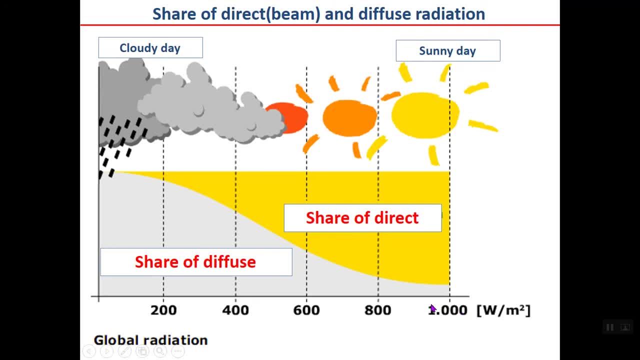 I want to remember you here That solar constant, Which was the solar Intensity on a surface Perpendicular to the sun rays And Outside the atmosphere, Or neglecting the atmospheric Effect, Is 1367.. Watt per square meter. 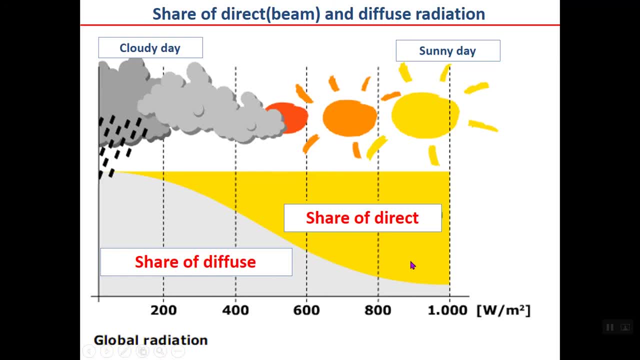 On average. Please remember this value also. This is Just a rough value, Because sometimes These values are needed For us as engineers. The solar intensity, Or solar irradiance At a completely sunny day, Okay- Is around 1000 watt per square meter. 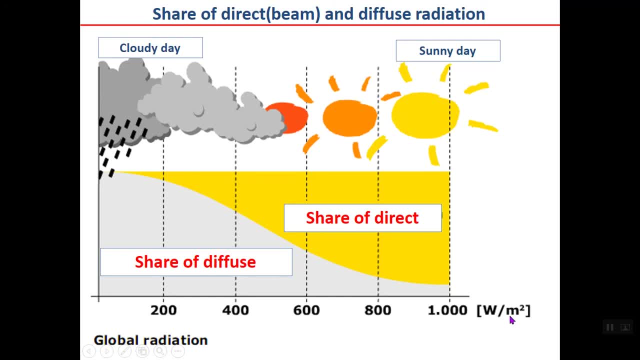 And don't forget That it cannot be More than 1367. Because that value Was the value Neglecting the atmospheric effect. So, as you have In real cases On the earth, So the value of solar intensity. 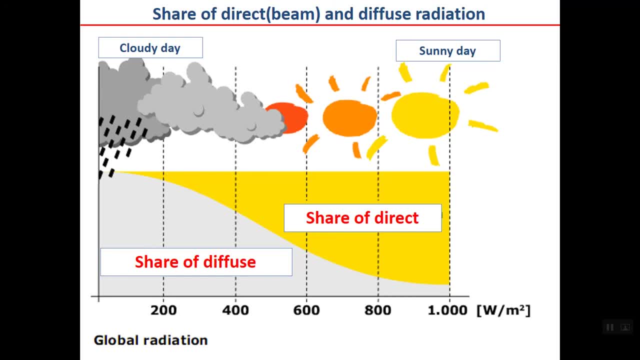 On the earth Will be always Less than 1300 or so Watt per square meter. You may remember 1000.. As a good estimation, A rough estimation For the solar intensity At the noon time, For example, In a sunny day. 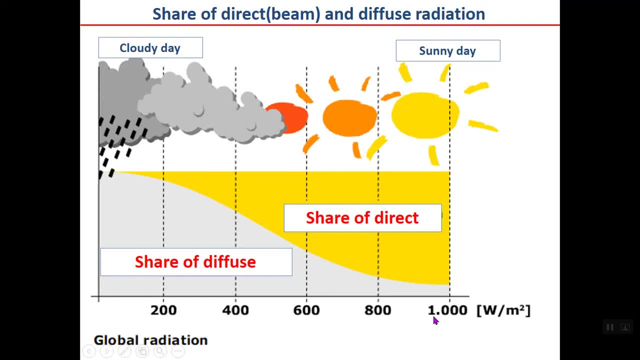 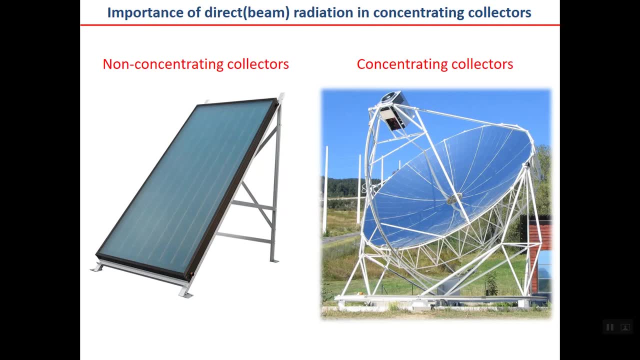 It is much more From me That you can use this value As an estimation For a sunny day. Okay, What is the importance Of direct radiation In concentrating collectors? Just an introduction. We will discuss About all these. 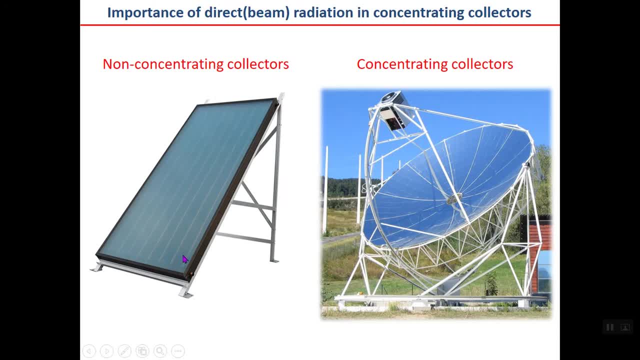 Later in more detail. But you have generally Two types of solar Receiving surfaces: Of the non-concentrating type. This means that the Sun rays are not concentrated. But you have also Concentrating type of collectors. There are different types of 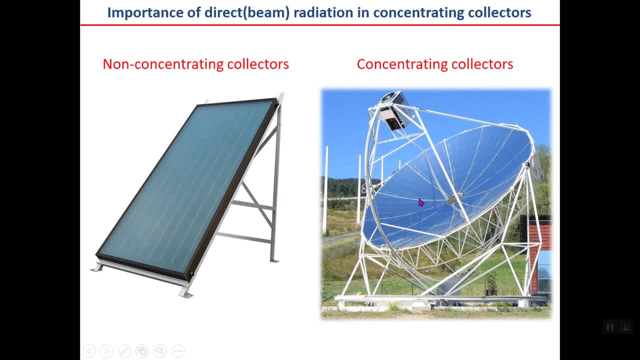 Concentrating collectors. At least there are four types. This is a dish sterling type, There is also Parabolic through collector, There are solar towers And also there are Fresnel collectors, Which we will discuss about them later, At least as a representative. 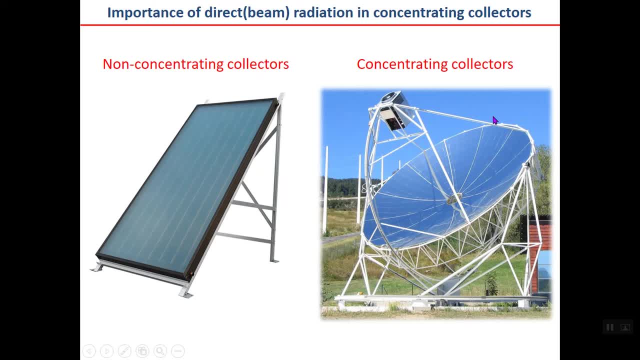 For the concentrating collectors In this type, as you can see, Solar rays hit the dish And then will be concentrated here. That, for example, sterling motor May be placed here to produce power. Okay, So you have non-concentrating type of collectors. 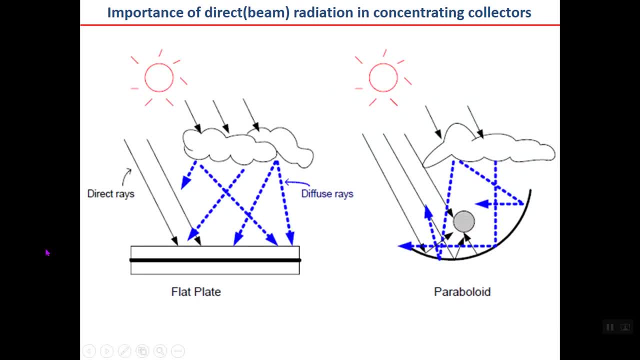 You have concentrating type of collectors. Okay, And what is the importance of Distinguishing between direct and Diffuse solar radiation? The important point here Is that for the flat plate Or non-concentrating type of collectors, They may work. 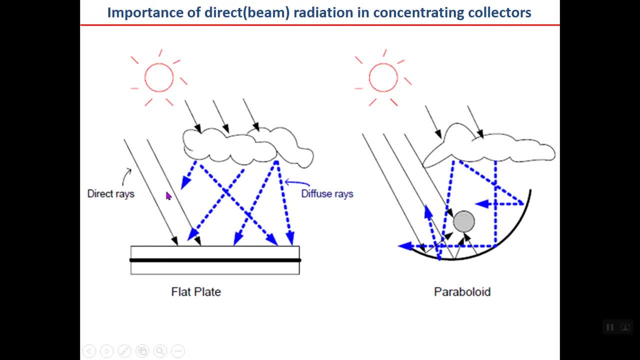 Both with the direct and diffuse rays. As you can see, Certainly the value of direct rays Will be, the share of direct rays Will be much more, But they also work with the diffuse rays. Okay, This means that, for example, in a cloudy day, 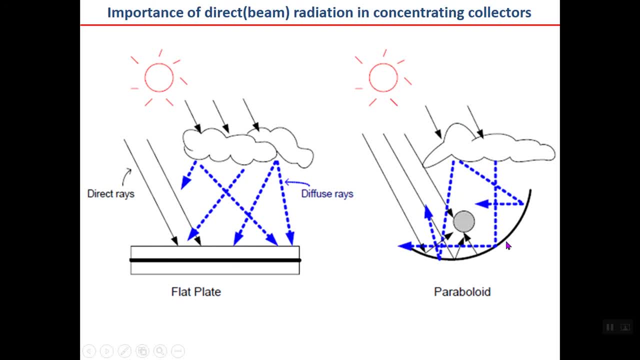 The output of the system is not zero. It has some output. But for the concentrating type of collectors, Like the parabolic Or something like this, You can see that these blue dotted lines Which show the diffuse solar radiation Cannot be concentrated. 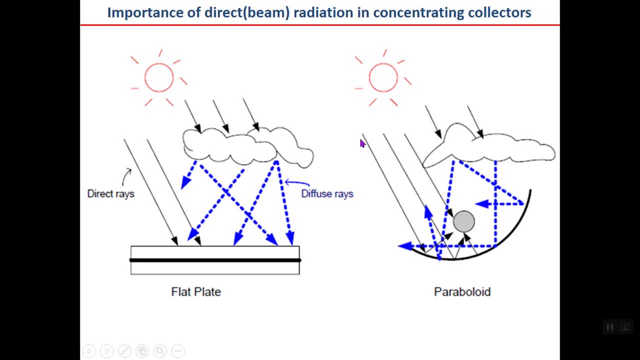 Or reflected to the tube Which is placed here. You can only reflect and concentrate Direct sun rays. For example, you may remember That in a cloudy day You cannot reflect the sun rays by a mirror. Okay, So for concentrating types of collectors. 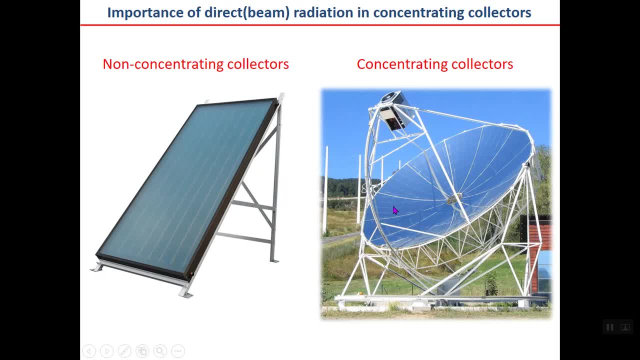 Like the one you can see here. D and I is very important, And so you can conclude That these types of collectors Or systems Can be installed only in locations Where there is a good direct solar radiation, And they cannot work. 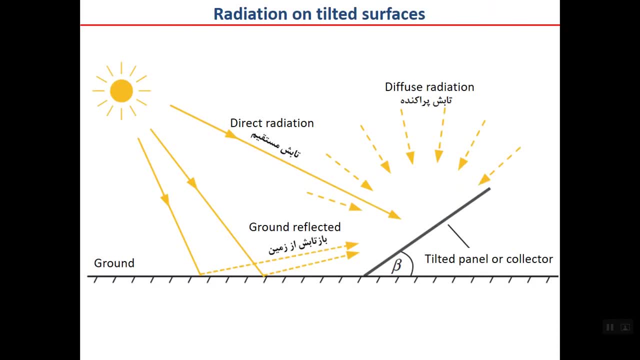 With diffuse solar radiation. Another important point here Is the distinguishing between Tilted panel or collector, Or horizontal collector or panel. Okay, Up to now We just discussed about The horizontal surface. The surface may be A solar thermal collector. 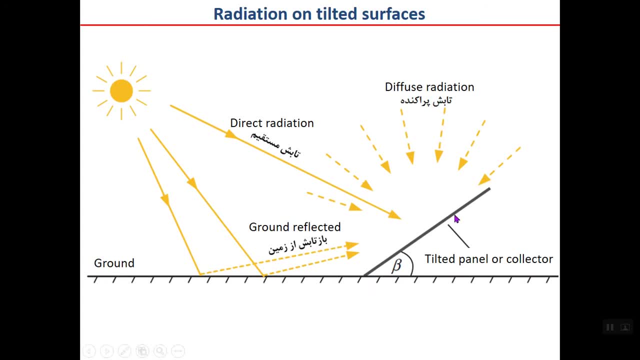 Or a PV module, And when you have a horizontal surface Then the total solar radiation On that is Includes just diffuse And direct solar radiation. But when the surface is tilted At an angle to the horizontal, Then there will be a third one here. 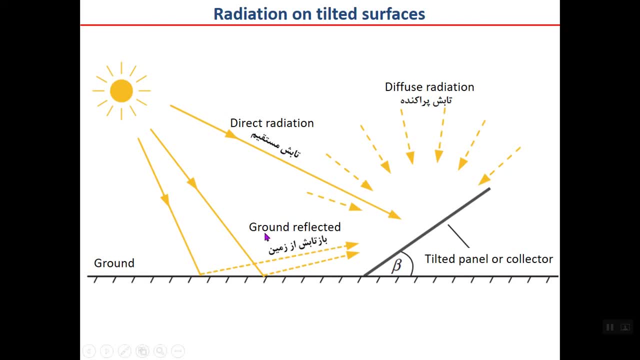 This is the ground reflected. What is the meaning? Ground reflected? This is the radiation Which, after hitting the ground, Reflects again to the surface That you have, Which depends On the type of surface And the surface color, For example. 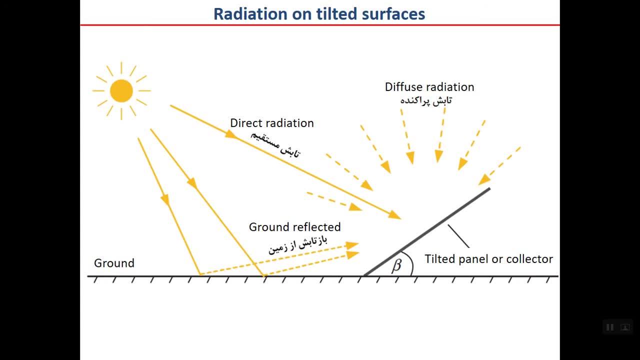 There is a difference between the grass, For example, Or a surface covered by snow Or any other Any other Desired surface. Okay, Let's just remember That it includes The share Of these three radiation Diffuse direct. 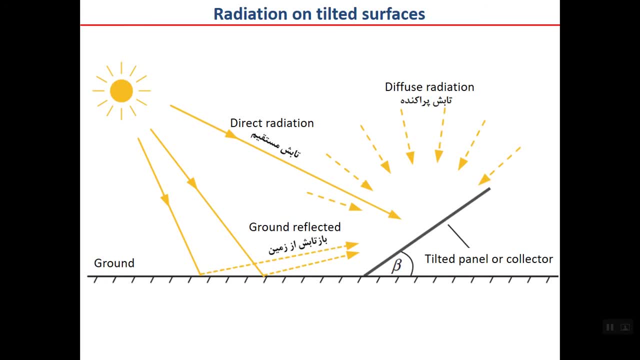 And ground reflected, But for the horizontal one It includes direct And diffuse solar radiation. I do not use the word summation Because you can see later That it is not so simple That just add, for example, Ground reflected to direct radiation. 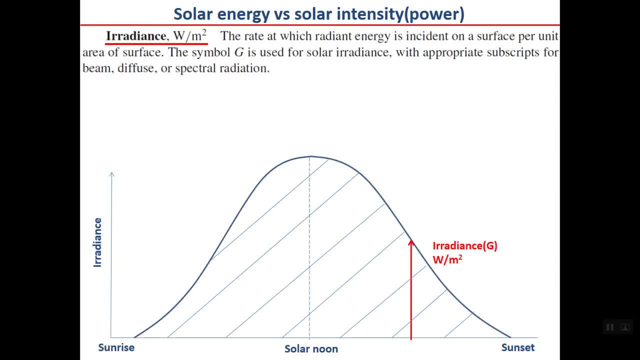 To diffuse radiation And diffuse solar radiation And diffuse solar radiation. The next And I think the last definition Is, or two definitions, About the irradiance And irradiation. We used these parameters before And I want to define them. 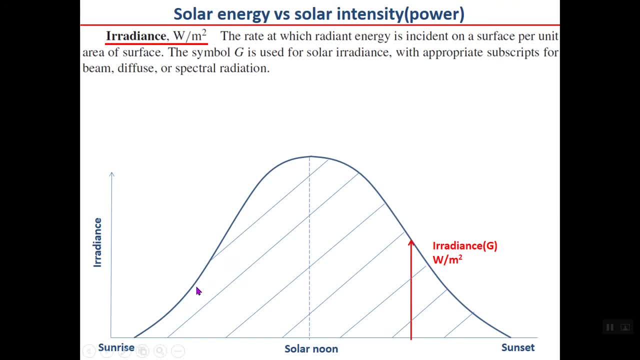 In a more specified manner. Now. This graph shows the variation Of solar intensity. Okay, Up to now, In the scientific world, Which is irradiance, The solar intensity starts at zero At the sunrise And if it's a sunny day, 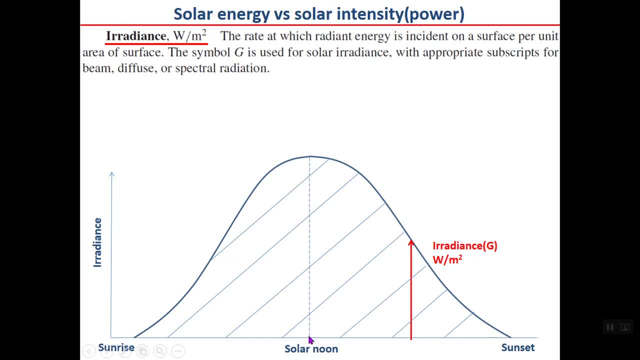 It will increase to a maximum Which occurs on the solar noon. Solar noon is not 12 o'clock. We will discuss about that next week. It's the time, The middle of the day And, as we know, Time of Adhan. 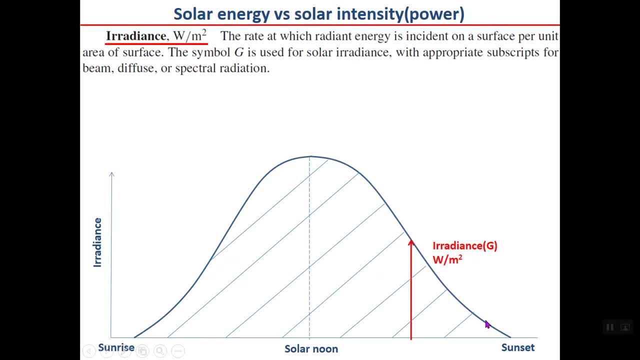 Okay, And will decrease again To the sunset, Where the solar intensity is zero At each moment of time. The instantaneous value Of the solar intensity Is named irradiance. Please repeat: Irradiance, Okay. In this book, 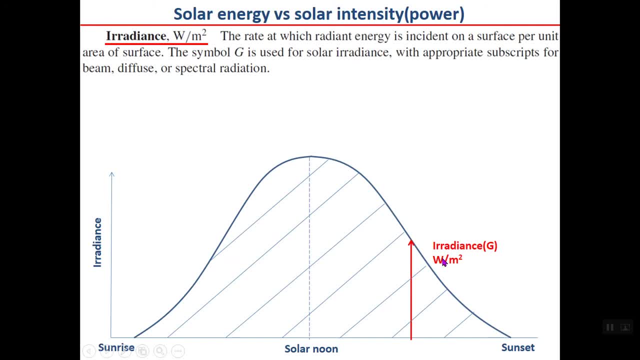 We will show irradiance by g. The unit is watt per square meter Or any other appropriate unit, And this denominator Shows the area, So the rate at which radiant energy Is incident on a surface Per unit area Of the surface. 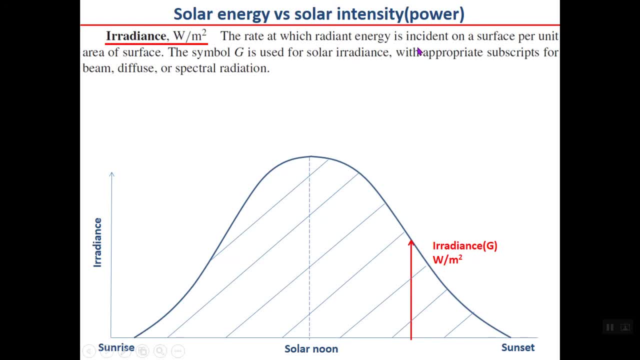 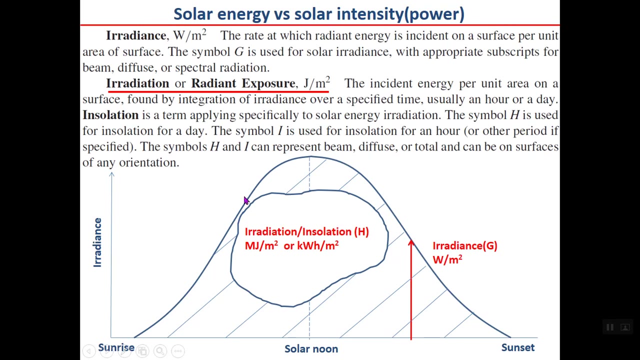 The symbol g is used for solar irradiance With appropriate subscripts For beam, diffuse or spectral radiation. What's the meaning When you put a subscript here, For example d, Then the meaning is diffuse irradiance. Okay, But The area 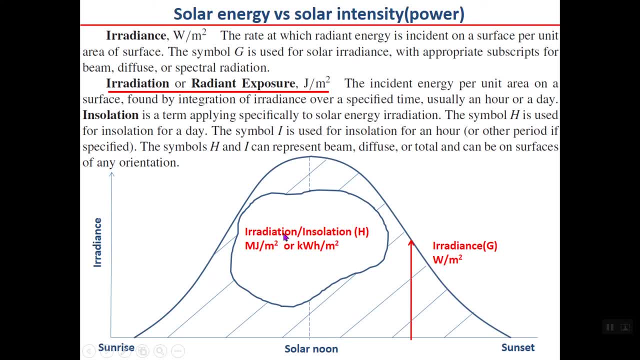 Below the curve of irradiance. You will give another parameter, Which is named irradiation Or insulation, Which is shown by h. Let's review the definition. The incident energy Per unit area on a surface- Please note this- is energy. 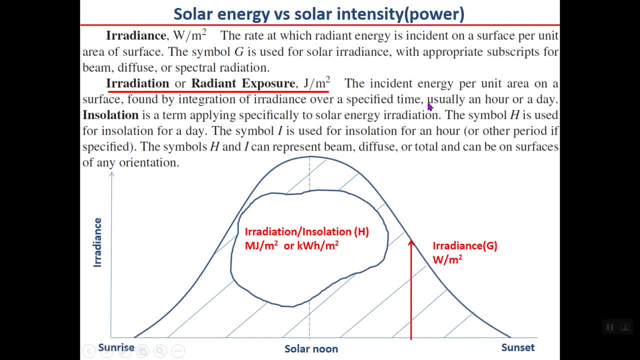 Okay, This is energy, But this one was rate Found by integration of irradiance Over a specified time. The name is insulation. Insulation is a term applying To solar energy radiation. If you integrate over a day, Then the symbol h 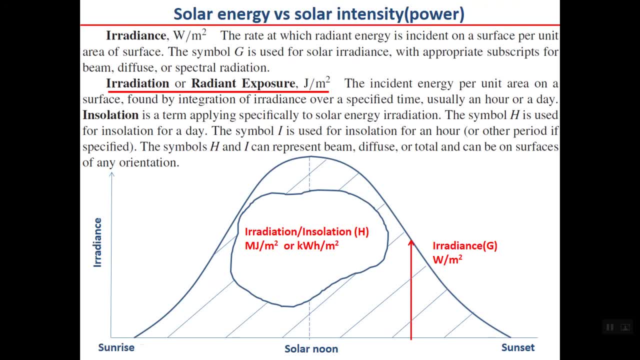 Is used for insulation for a day. Okay, So whenever you see h, It is the integration of the area Below the curve from sunrise to sunset. But if You see symbol i, The meaning is that It's not from sunrise to sunset. 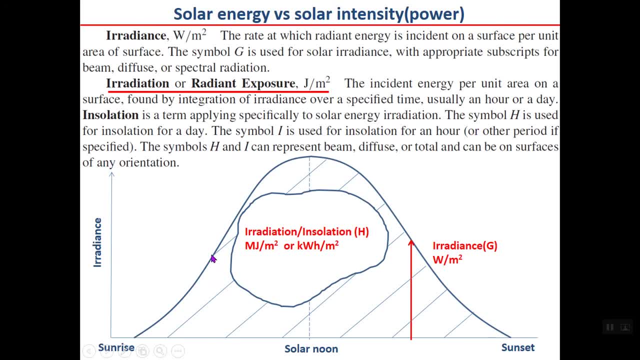 It may be during any Time, For example from 9 o'clock to 10 o'clock. The symbols h and i Also can represent beam diffuser Total By the appropriate subscripts And can be on Surfaces of any orientation. 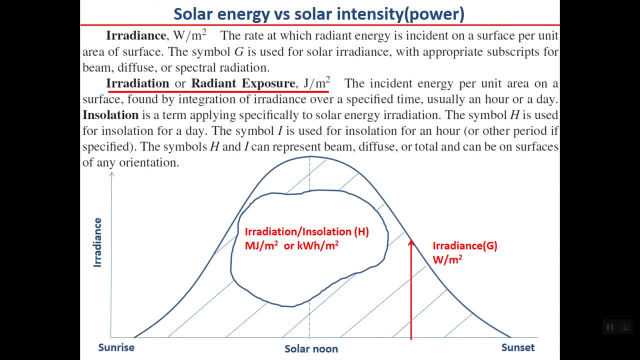 It means that it may be horizontal, It may be at an angle, Tilted or it may be To any direction. The unit for h, as you can see, Is joule per square meter Or watt hour per square meter, And it is used generally. 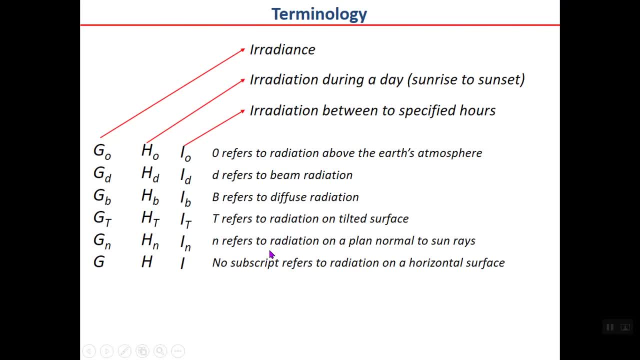 So become familiar with Both of them. In summary, We have three parameters: g, h and i. As I told you, g is irradiance. h is irradiation during a day, Sunrise to sunset. i is irradiation between two. 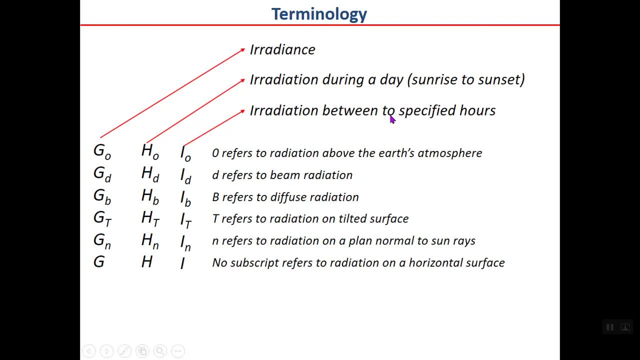 Sorry, it is not t o, It is t w o- Two specified hours. Okay, The subscript, as you can see here, Has different meaning. For example, if you have t, This refers to the irradiation On a tilted surface. If there is no subscript, 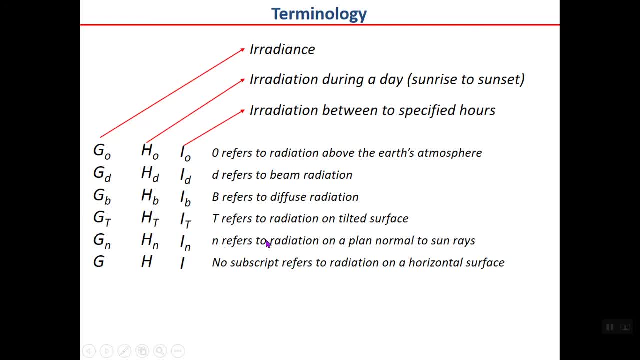 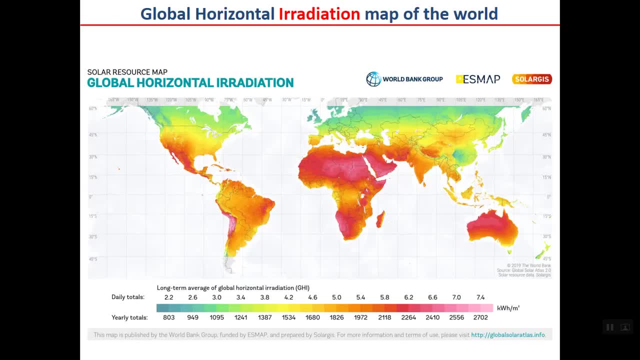 Then it is on a horizontal surface. If it is n, It refers to the irradiation on a plane Normal to the Sunrise. Okay, Global horizontal irradiation values Are generally You can find in different websites, Like the one you can see here. 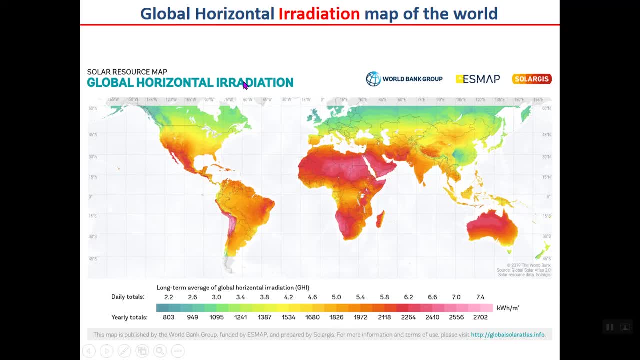 For example, this is the distribution Of global horizontal irradiation. You remember that g, h, i Is the irradiation And you know the difference Between irradiation and irradiance. Irradiation is the energy Which is integrated over a day. 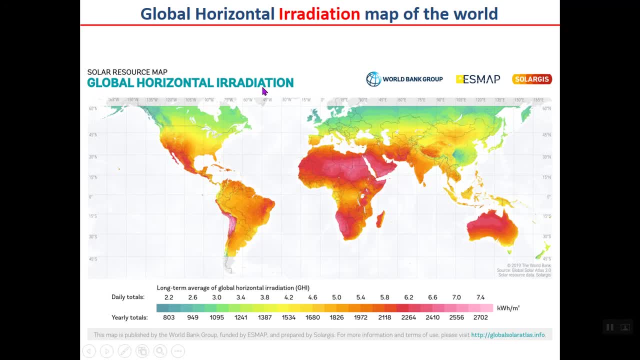 For example, Irradiance is rate. This graph Is the irradiation And actually tell it frankly, We generally work more With the irradiation Instead of irradiance, Because irradiance Is an instantaneous value And has no much. 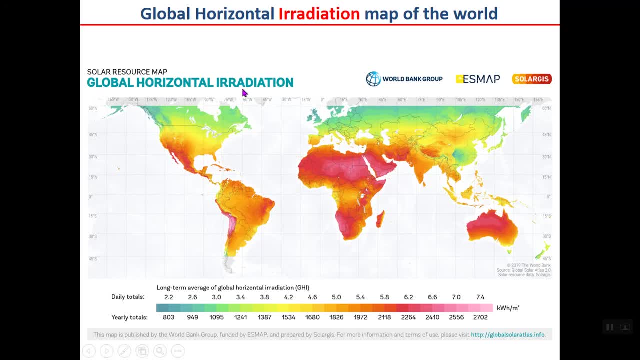 Use in our work. We generally work with the irradiation Because it is more useful for us For our calculations. Okay, You can see here that. Here the legend, For example, the colors Show the value of irradiation: G, h, i. 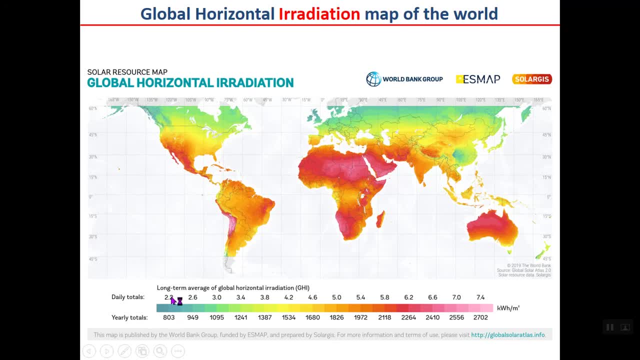 And the bottom ones Are the yearly totals. Actually, the yearly totals Are the daily Multiplied by 365.. And the value, as you can see, Is kilowatt hour per square meter. The daily totals Are an important one. 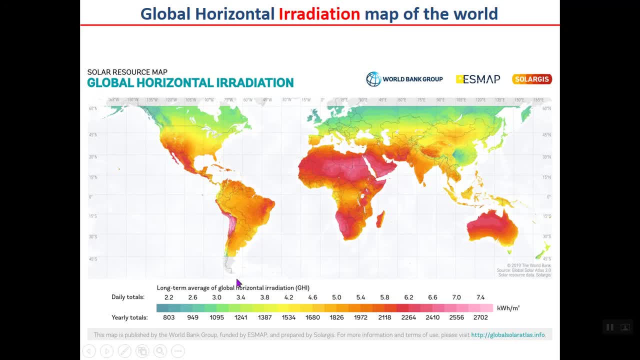 Because there We have another parameter Names p, s, h Or pixon hours a day, Which we use for designing Photovoltaic systems. We use them in our work, Thank you, Okay, I will let you guys Please note to the values. 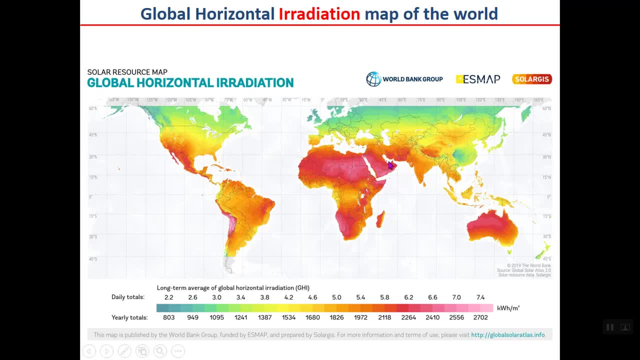 And we will discuss about that. Okay, Come to the graph. For example, here, In different parts of the world, You can see the value of solar irradiation. It may be interesting for you That, for example, in Iraq, In comparison to other points, 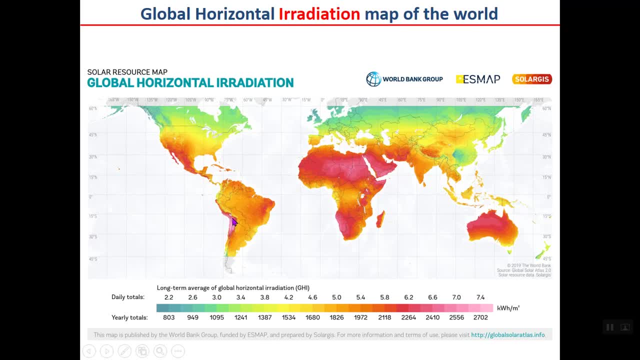 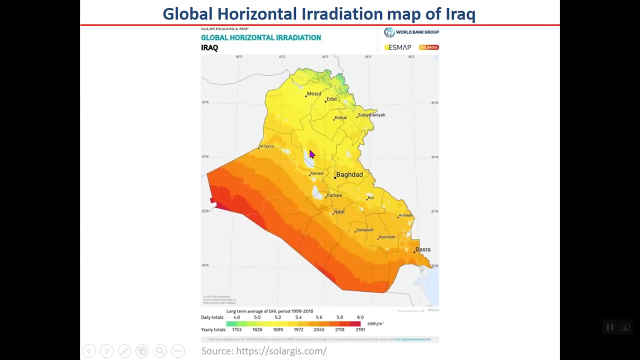 Or other locations in the world, or here in the America or some parts in the south of Africa and here at the north of Australia. but but again it's a good value in comparison, for example, to Turkey or in to the, to the Europe or many other places in the world also. it is possible to have a specific solar radiation. 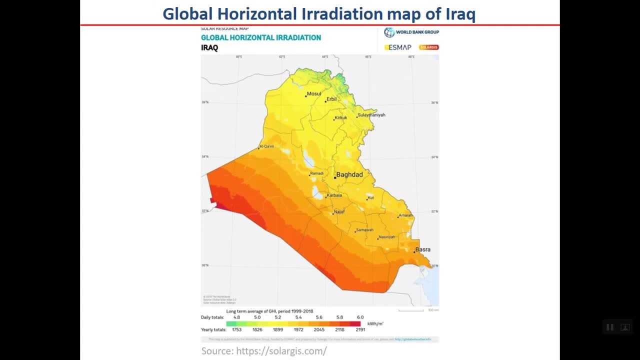 global horizontal irradiation maps for any specific country or region. for example, this is such a map from solargiscom, which we will see together just now. as you can see, for example, in Iraq you have the maximum global horizontal radiation in this area in the southwestern. 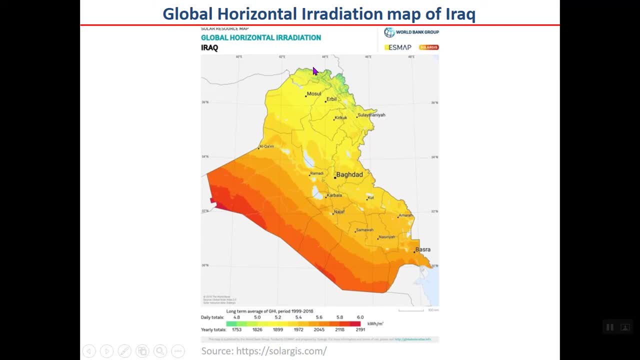 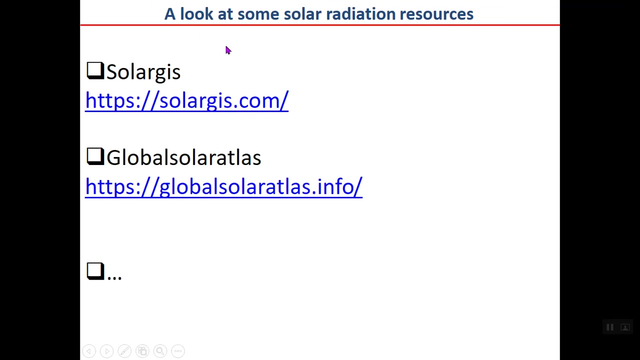 area of Iraq and the minimum value in the northern part and the northeast part of Iraq, and each color here shows a value. where you can, you can say what's the value referring to the legend. okay, let's now have some. have a look at some solar resource websites. there are a lot more. 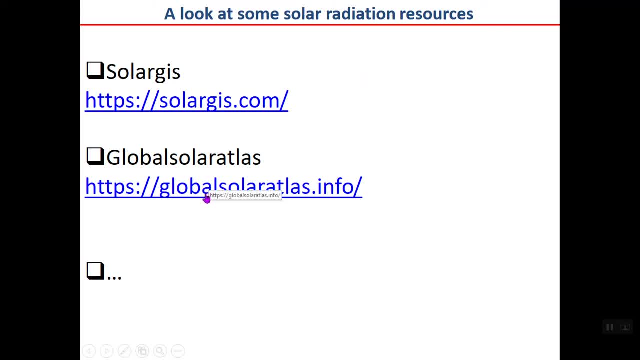 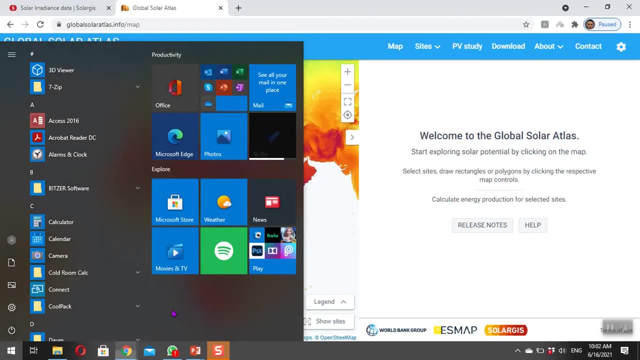 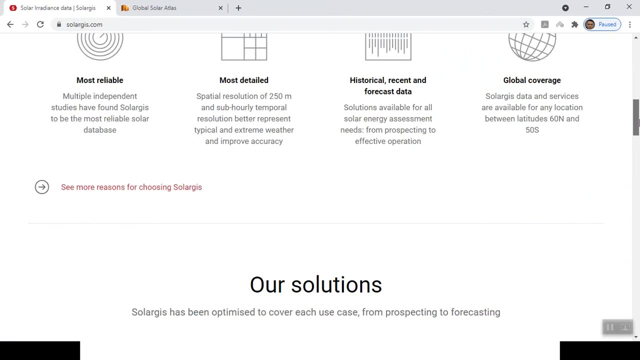 I want just to show two of them: solargiscom and global solar atlas. let's have a look at these two websites. okay, the first is solargiscom. here you can see there are a lot of information in this website. you can go through the details. 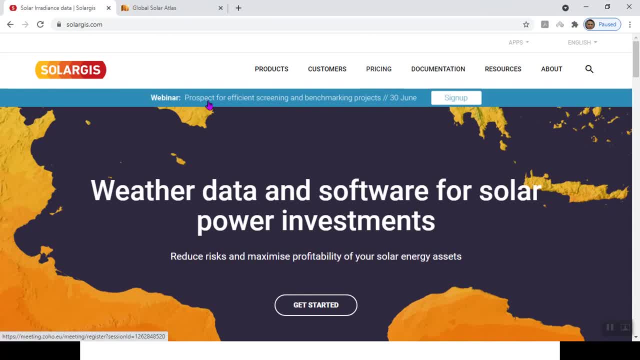 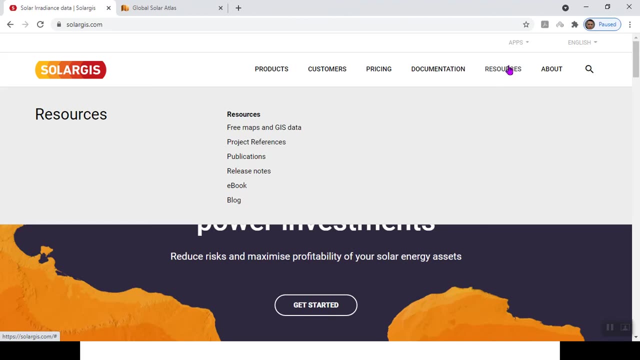 and also there are webinars, as you can see. the next one is prospect for efficient screening and benchmarking project on 13th of June, but for now I just want to show you one important resource here. click on resource. there's a tab on the above and when you are clicking on resources, then you 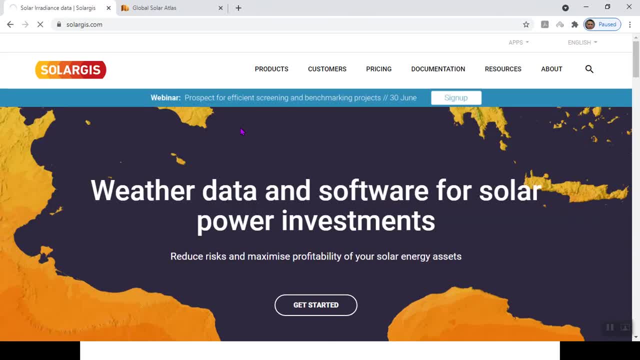 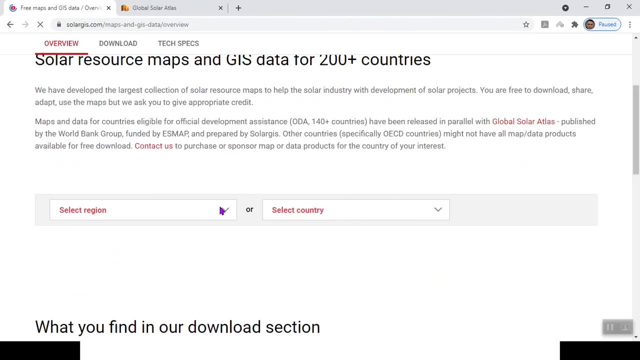 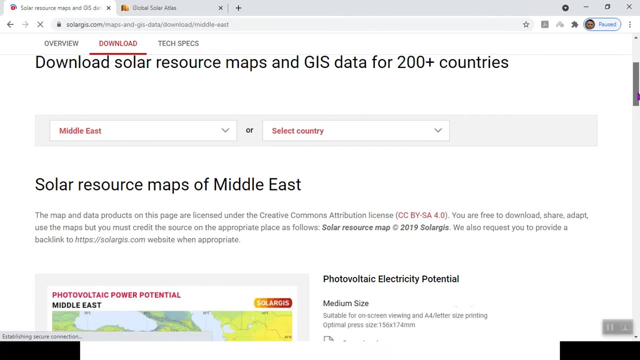 can click on free maps and gis data, for example. there are much more in this website, but I just want to show you one of the capabilities. this is the solar resource map. select the region. for example, here you can select Middle-East. wait for the page to be uploaded and then you can select. 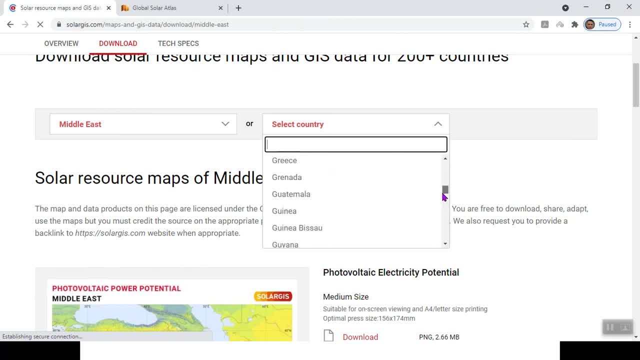 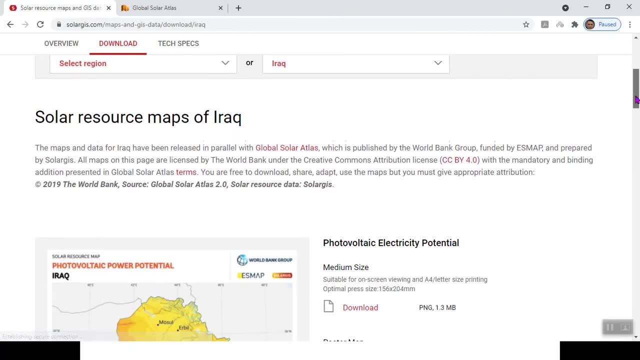 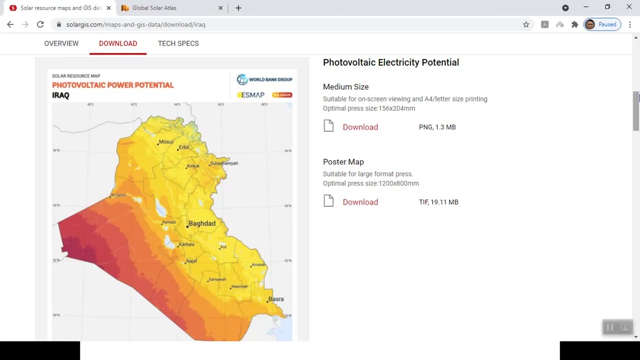 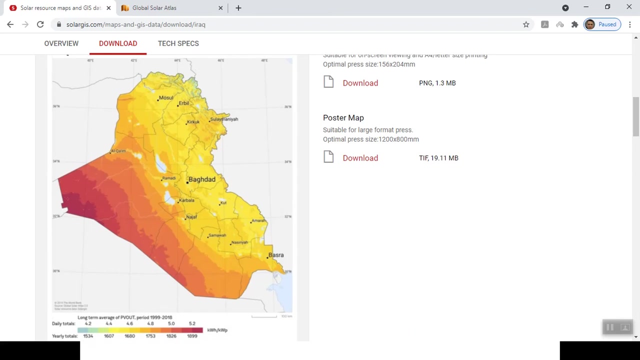 your country, for example. you may select, for example, Iraq, again, just for the page recommendation to be uploaded again, and you can see here different maps, for example. the first one is the photovoltaic electricity potential. this we will discuss later, but just to have a short introduction to what is this graph. it is kilowatt hour per kilowatt. peak kilowatt hour mean the 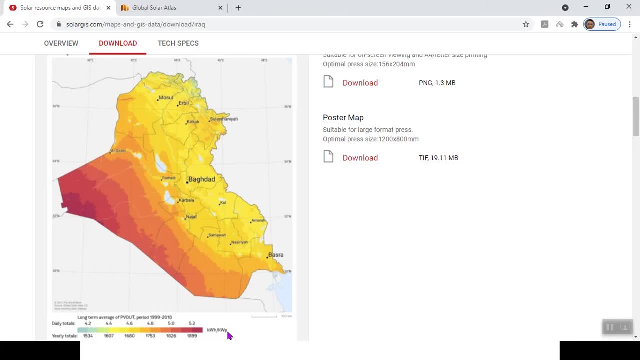 energy produced. kilowatt peak is the peak panel or nominal power of the photovoltaic panel installed. this means that, for example, in this area, in this specific area referring to this color, per day, for example, five kilowatt hours of energy is produced per kilowatt panel installed in this. 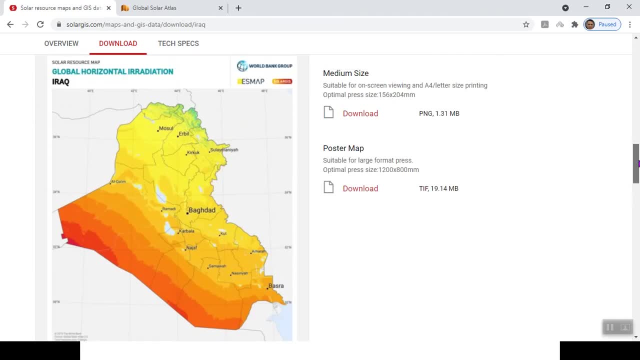 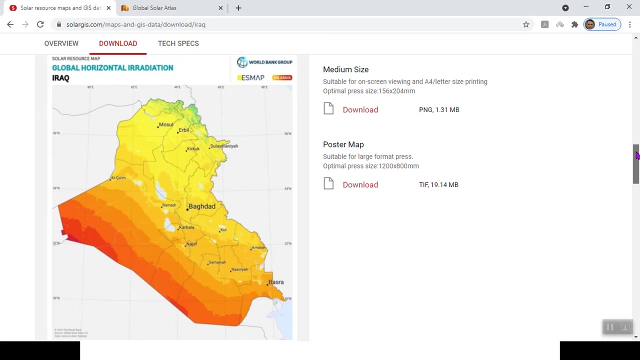 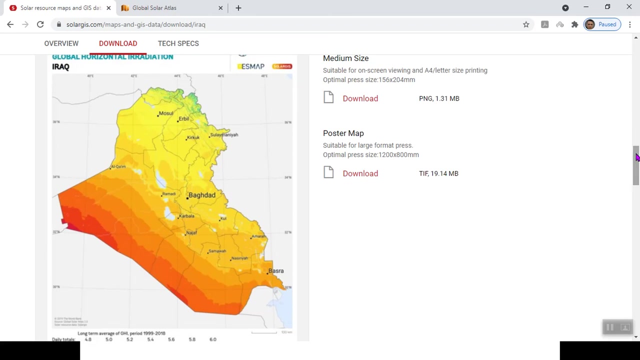 area. we'll discuss about that later. this is global horizontal irradiation, which we discussed just now. you can download the map, as you can see here, either in a medium size or a poster map. i advise you to download the map and print it in a full size and stick it in your room, and then everyone who see the map can distinguish that. 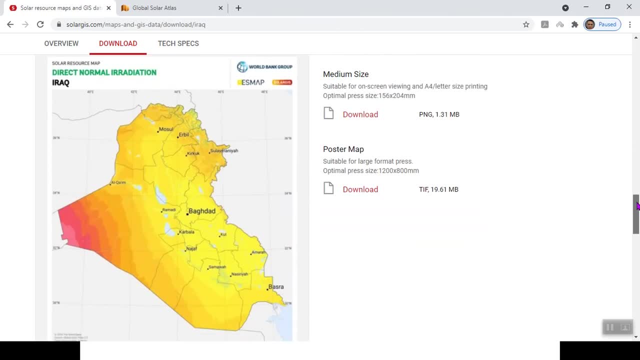 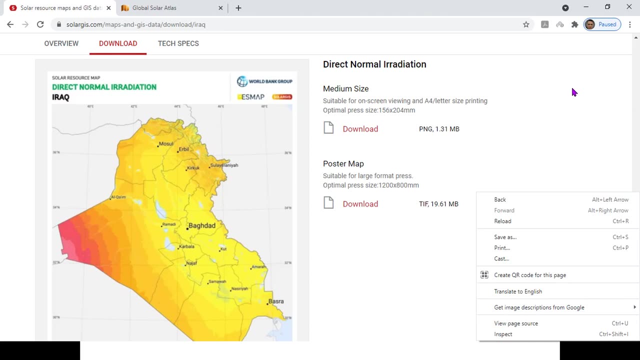 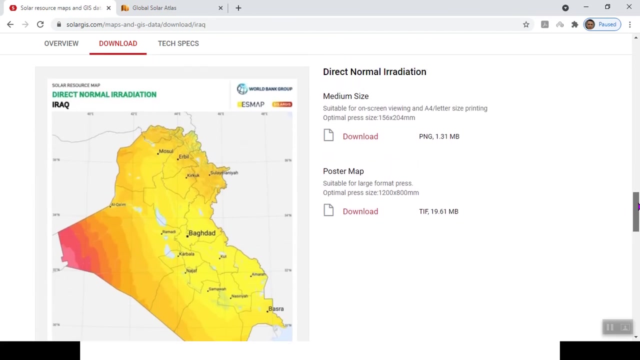 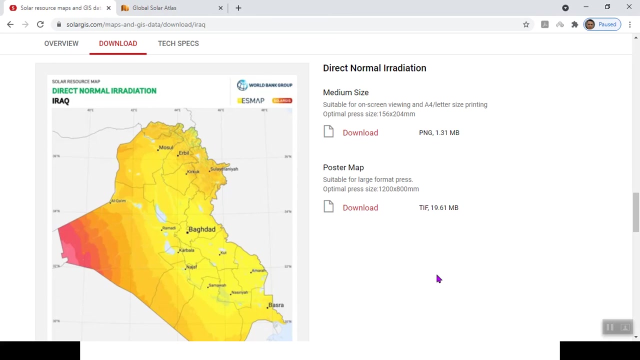 you are a fan of solar energy. this is a good idea to make your brand on solar energy, starting from here, putting a big map of your country solar energy potential in your room, either in your home or office. okay, this is the map for the direct normal irradiation. you remember that this was also one of the parameters in solar 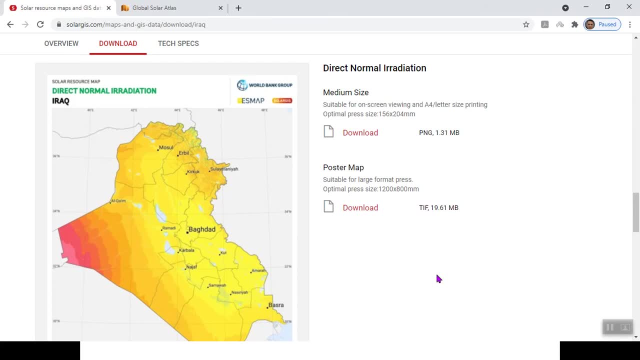 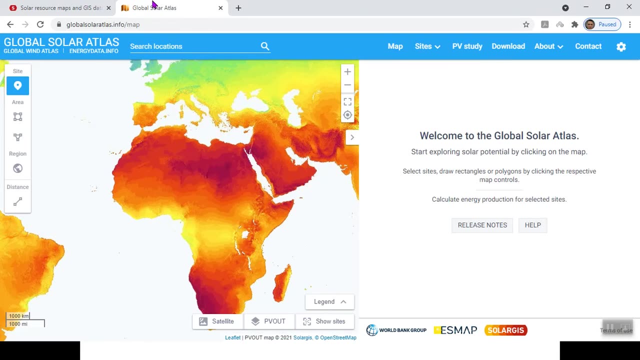 energy: direct normal irradiation. again, you can see the variation of dni over the country. the other website here you can see is the global solar atlas info. it's a very, very informative website with a lot of possibilities. i want just to show you one of the them here. at the beginning you can see a map. you can see what is showing in the map. for example, if 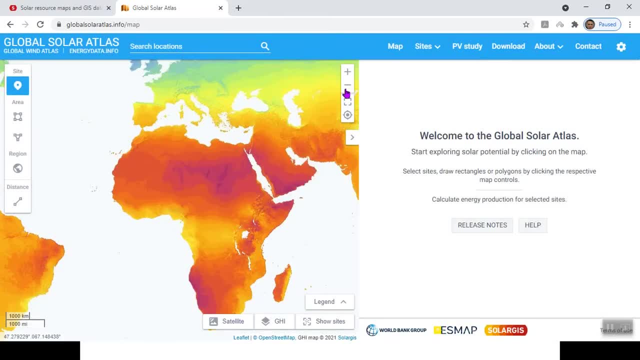 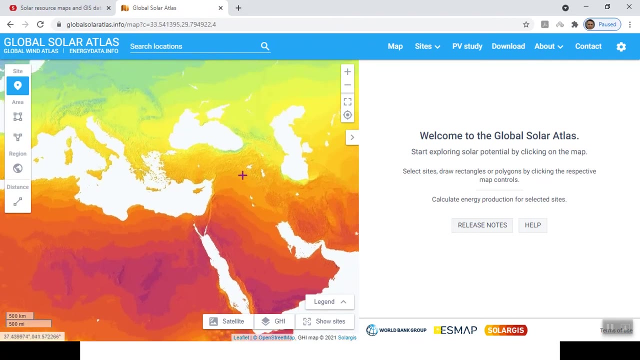 i want to show global horizontal irradiation. i choose that you can see the world map as you can see here, or you may zoom in or zoom out for a specific area. for example, if you put your mouse on an area and click on that, then here you can see that, for, for example, it's in. 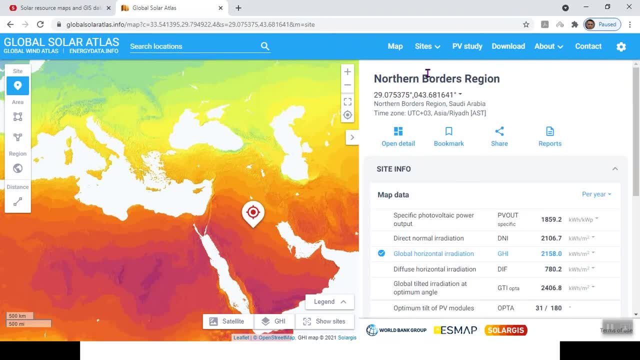 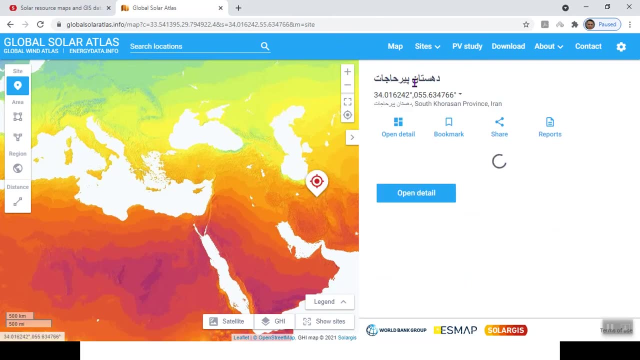 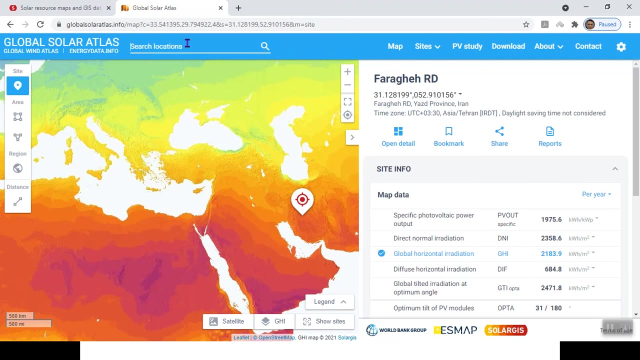 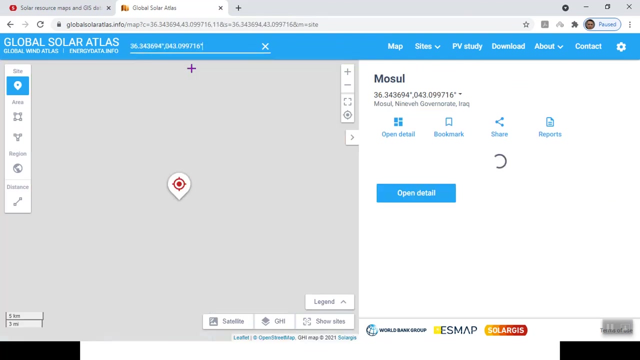 mediat in turkey or, for example, here, it is in northern border region, here, for example, it is in libya, or here, for example, it is in somewhere in iran, or here or here, or you may type the name of the location. for example, if you, for example, tag muscle, for example in iraq, then click on that. 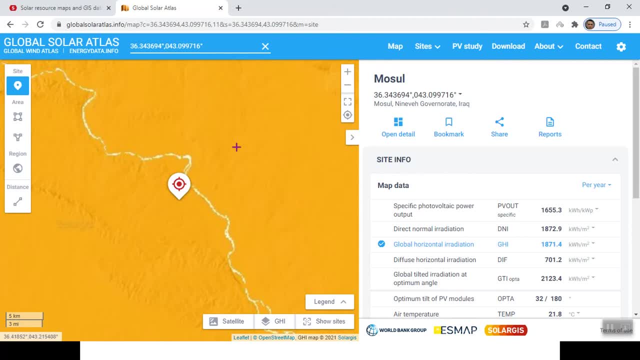 it goes to the location, you can again zoom in and zoom out. you can also select different. do do work with these different items in the website. i leave it to you to do that. okay, then you can see, for example, in mosul in iraq, you can. 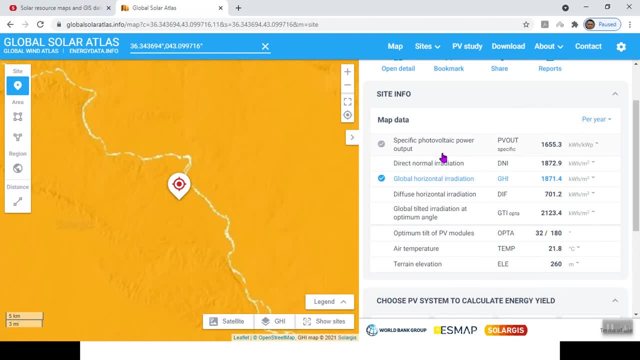 see here different parameters. i think if you are using a mobile phone then it's the table may be shown. uh, below the the map. i don't know, you can check it yourself, but you can find it somewhere. finally, okay, here you can see the global horizontal irradiation. you can see that, for example, for muscle global. 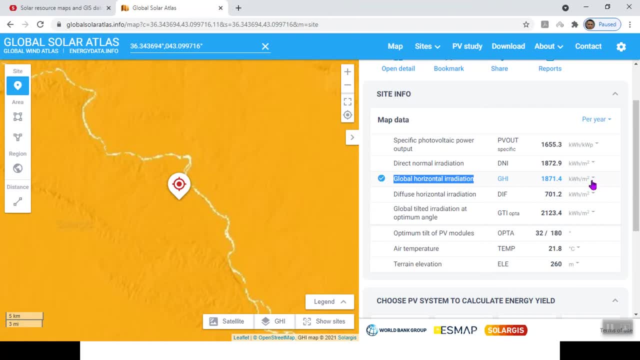 horizontal irradiation is 1871 kilowatt hour per square meter per year. you can change this to per day, for example. then it will be 5.1, or here you can change also the units, as you can see. it may be kilowatt hour or mega joule per square meter. here you can see the diffuse horizontal irradiation. 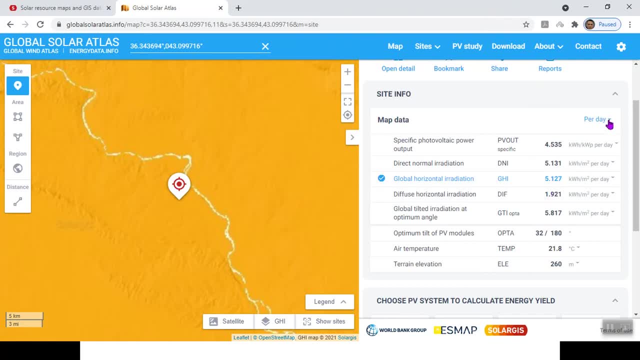 or diff, which is 19 per day. let me change it to per year, okay, and then here you can see that when you click on some of them, the color will be also different. actually, it goes to: for example, this is dna, when, i please note, this is dna. and when i click, when i click on global horizontal irradiation, it will show the. 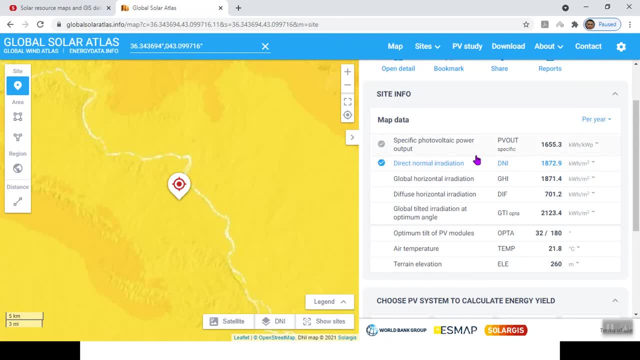 ghi global result of irradiation. dna, as you remember, is the direct normal irradiation, which was the radiation on the surface that is directed normal to the. it is placed normal to the sun rays and it is 1800, as i told you before. please note that the 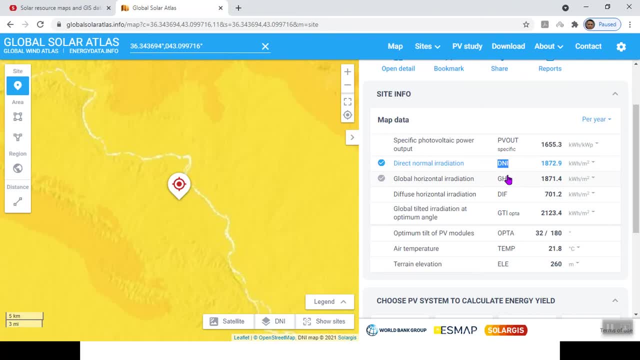 sum of diff, or ghi, and dni is not equal to ghi. it needs a correction for the zenith angle of the sun. okay, you can see other parameters we will discuss about later, for example, solar photovoltaic power output. as i told you, this is the energy produced per kilowatt panel installed. 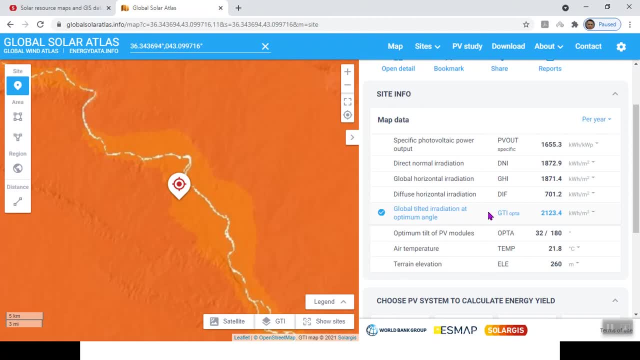 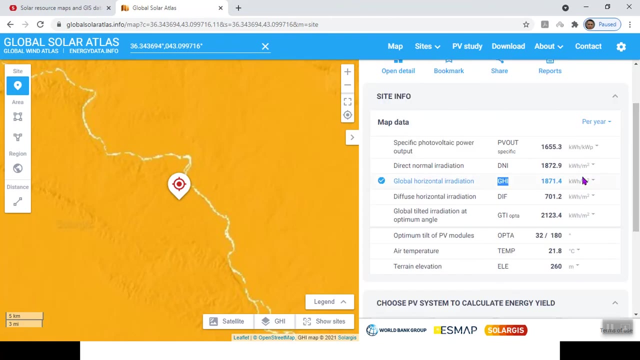 this is the global tilted irradiation and optimum tilt angle, because we told, i told you that gti, or tilted irradiation, is different from the ghi. okay, you can see that when you have, for example, horizontal surface in mussel. okay, the yearly solar irradiation or insulation is 1800, while 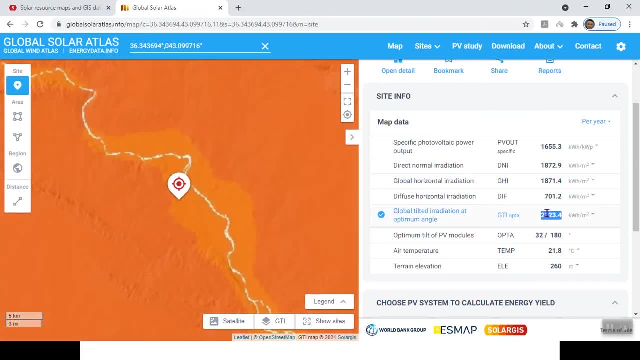 if it is placed on an optimum tilt angle, then the value will be much more. you can see it's 2000- 2001.. what is the optimum tilt angle? for example, based on the calculation from this website, the optimum angle for mussel is 32 degrees. what's the meaning? it means that, for example, you 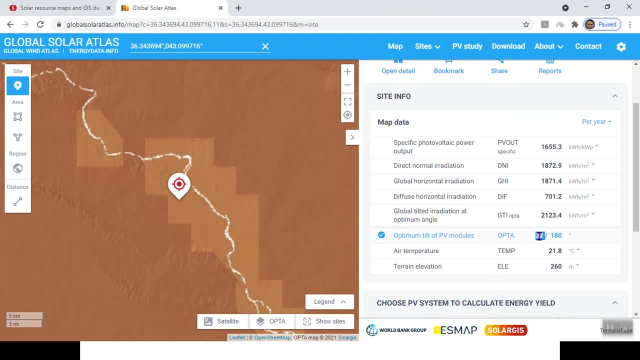 should place the panel at an angle of 32 with respect to the horizontal. what is 180? it is the optimum direction for this website. zero is taken as the salt, so sorry at the north. so 180 means that the panel should be directed toward the salt. what's the average air temperature? this, and the elevation is 260 meter. there are lots more in. 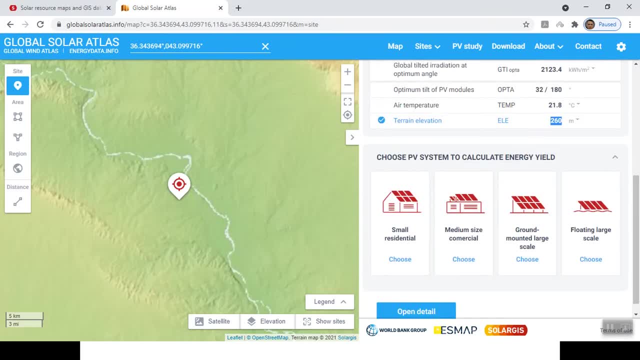 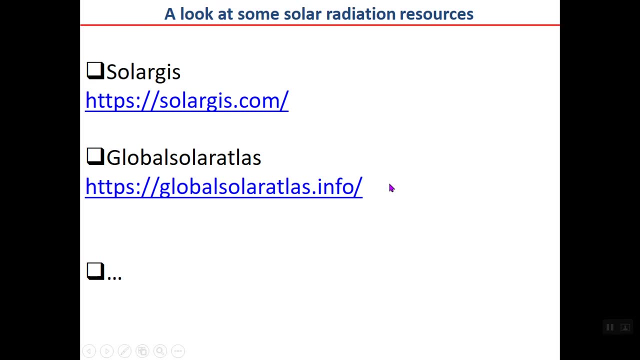 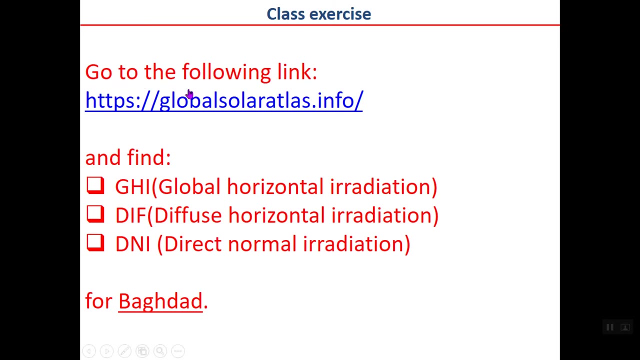 this website, for example, you can also choose a system to calculate, but i leave them either for you to you to do it later, or we may come back to this website again later. and this is an exercise: go to the same link and find ghi, diff and dni for, for example, another city like Baghdad, or